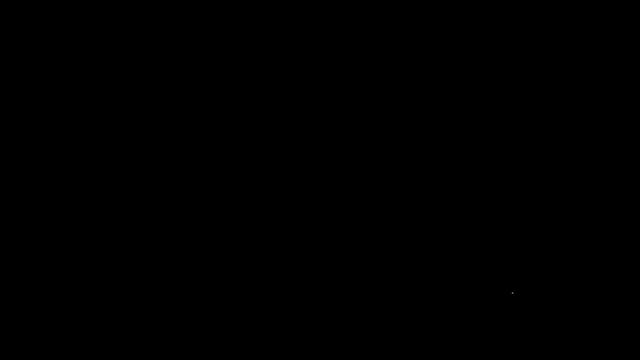 In this video we're going to talk about AC circuits and impedance. So the first thing you need to know is that the RMS voltage is equal to the peak voltage divided by the square root of 2, and RMS current is equal to the peak current divided by root 2.. Now let's say if we have an AC source connected to a 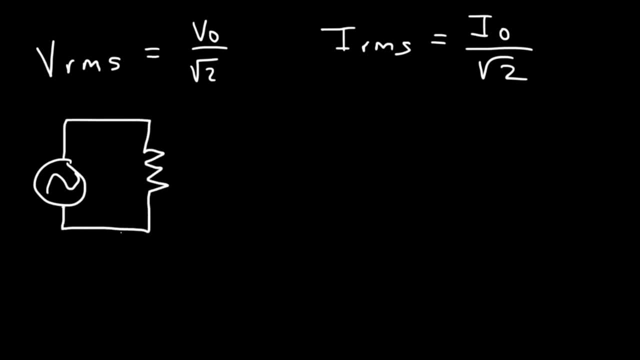 resistor. In this circuit energy is transformed into heat. The current and the voltage are in phase, So voltage is equal to current multiplied by resistance, and the average power consumed in the circuit is simply voltage times current. So let's work on the problem. Let's say, if we have a 120, 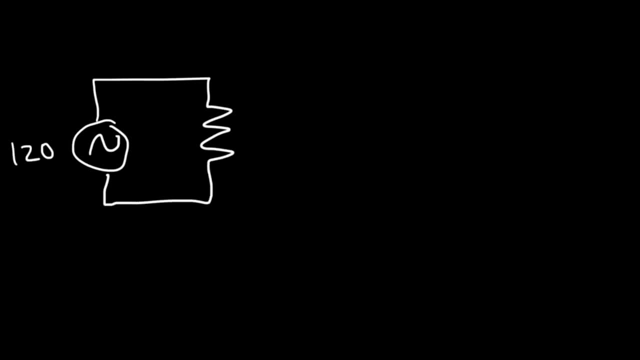 volt AC. So let's work on the problem. Let's say: if we have a 120 volt AC? So let's work on the problem. Let's say: if we have a 120 volt AC, Now let's say that the resistance is 100 ohms, What is the current that flows? 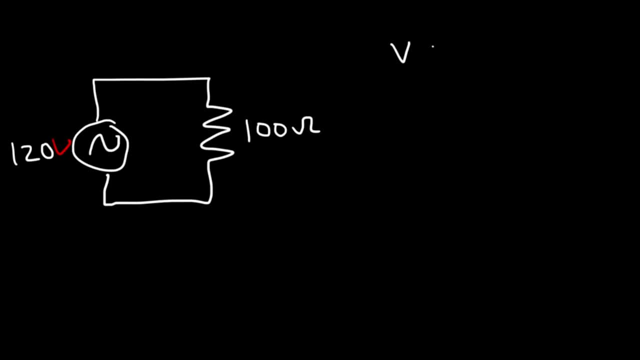 in a circuit. So, using equation, V is equal to IR, the voltage is 120, the resistance is 100.. So 120 divided by 100, the current in the circuit is 1.2 amps. Now how much power is dissipated by the resistor. 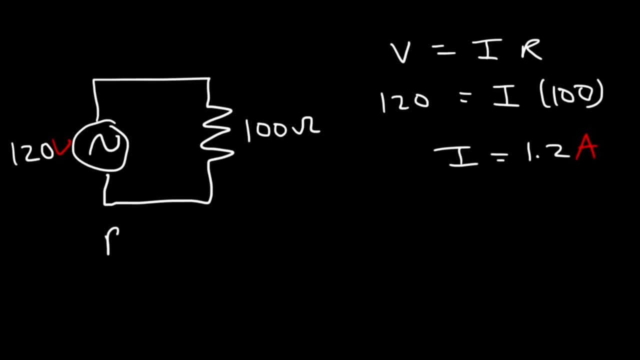 So power is equal to voltage times current. The voltage across the resistor is 120 volts and the current that it uses up is 1.2 amps. So 120 times 1.2 is 144 watts. Now let's say if we have an AC signal. 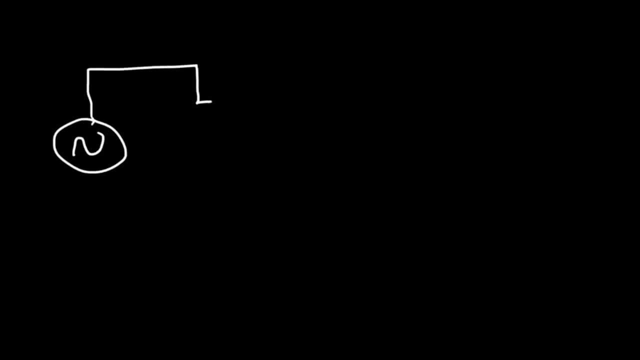 So 120 times 1.2 is 144 watts. Now let's say: if we have an AC signal, So 120 times 1.2 amps. Now let's say, if we have an AC signal, So 120 times 1.2 amps is 14 volts. First of all, we have to teach current vomiting. 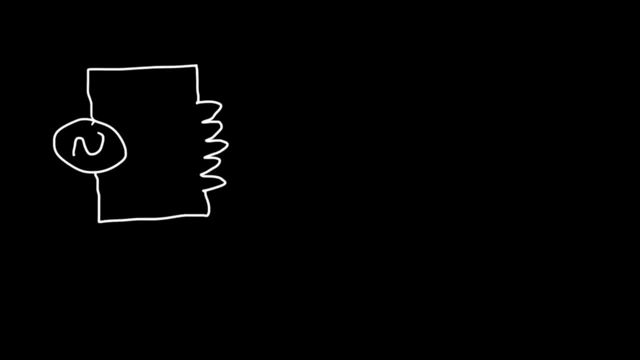 there. OK, Let's talk about Ο patient and assistance in this video. So now we have 전 current, that is, an alternating currentietached to an inductor which has this symbol. The inductor has the inductance, let's say 50 millihenries. 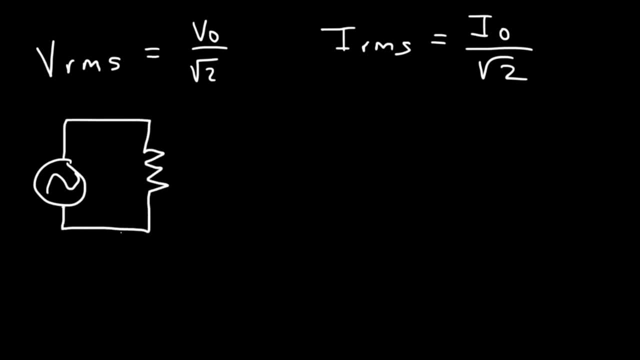 resistor. In this circuit energy is transformed into heat. The current and the voltage are in phase, So voltage is equal to current multiplied by resistance, and the average power consumed in the circuit is simply voltage times current. So let's work on the problem. Let's say, if we have a 120, 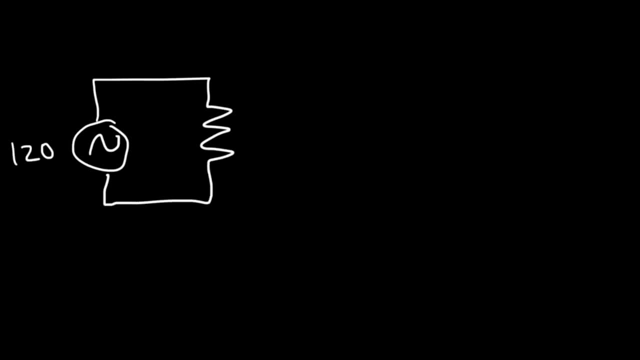 volt AC. So let's work on the problem. Let's say: if we have a 120 volt AC? So let's work on the problem. Let's say: if we have a 120 volt AC, Now let's say that the resistance is 100 ohms, What is the current that flows? 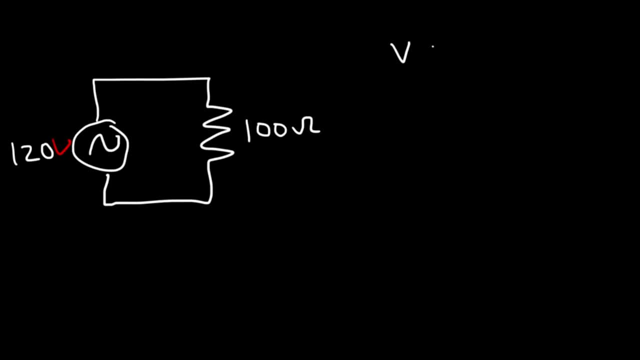 in a circuit. So, using equation, V is equal to IR, the voltage is 120, the resistance is 100.. So 120 divided by 100, the current in the circuit is 1.2 amps. Now how much power is dissipated by the resistor. 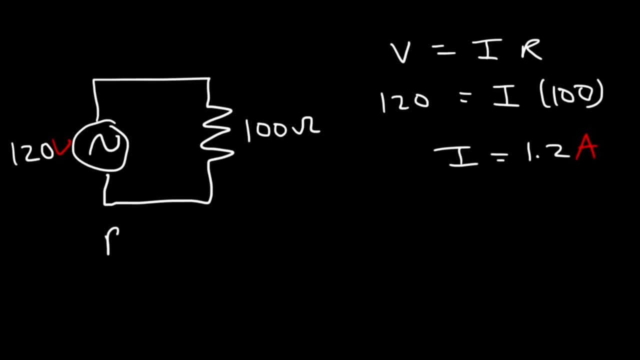 So power is equal to voltage times current. The voltage across the resistor is 120 volts and the current that it uses up is 1.2 amps. So 120 times 1.2 is 144 watts. Now let's say if we have an AC signal. 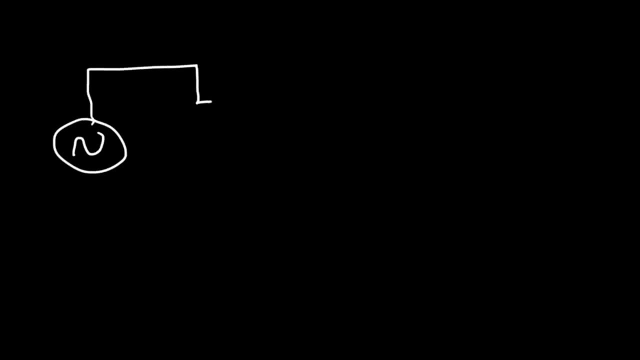 So 120 times 1.2 is 144 watts. Now let's say if we have an AC signal, So 120 times 11Hi we have the AC signal. we need to choose an AC current, that is is an alternating current attached to an inductor which has this: 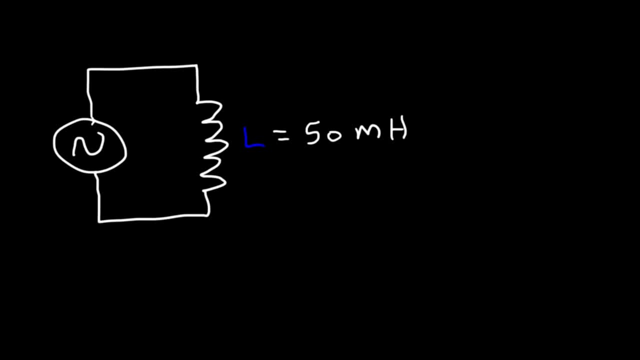 symbol. The inductor has the inductance of, let's say, 50 mH. What equations apply in the circuit? The inductive reactance represented by xL is equal to 2 pi fL. xL is measured in ohms, like resistance. 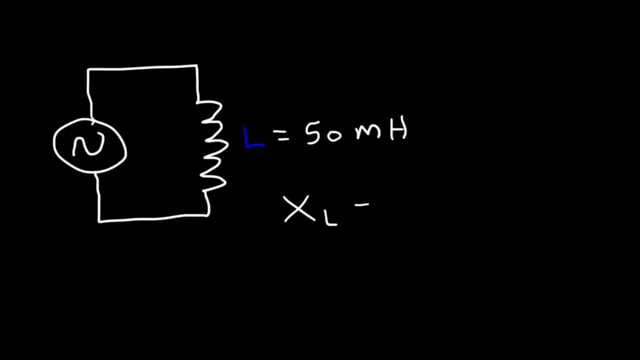 What equations apply in this circuit? Inductors present inductive reactance to an AC circuit which acts like resistance. The inductive reactance represented by xL is equal to 2 pi fL. xL is measured in ohms, like resistance. 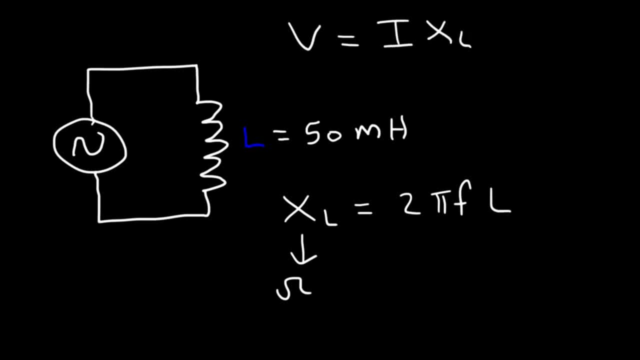 So, just as V equals IR, V is equal to I times xL. If you were to plot a graph between the frequency and the inductive reactance, these two are directly related. As the frequency increases, the inductive reactance increases as well. 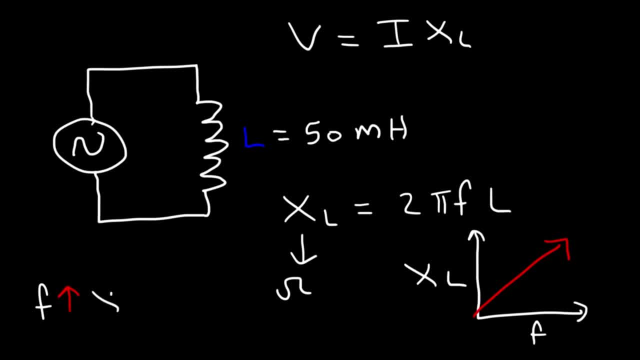 So when f goes up, xL goes up And as the inductive reactance goes up, the current in the circuit decreases. Current and inductive reactance are inversely related. So high frequency AC signals will yield less current in the circuit and low frequency 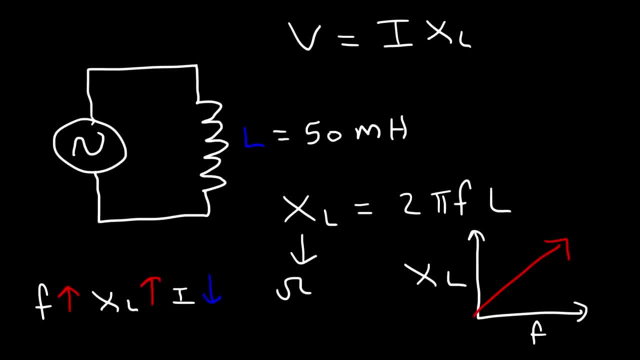 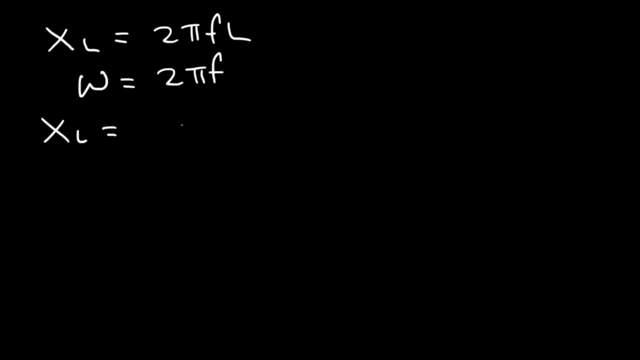 signals will yield less current. Now, going back to this equation where inductive reactance is equal to 2 pi fL, you need to know that omega, the angular frequency, is equal to 2 pi f, So xL can be represented as omega times L. So just keep that in mind. 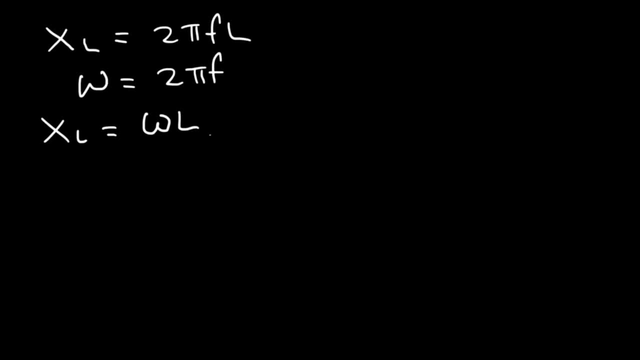 Also for an inductor, the current lags the voltage by 90. You need to know that as well. So that's it. Thanks for watching. See you next time. So whenever you have an AC signal passing through an inductor, the AC signal, the current. 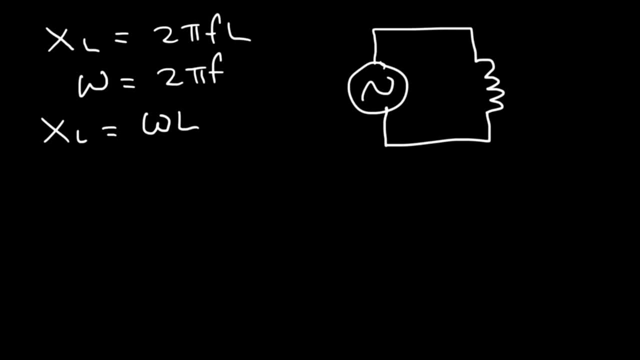 in. it is changing. It's increasing and decreasing. It's not constant And because the current changes you're going to have a change in magnetic flux inside the inductor. As the current increases, the energy stored in the inductor increases as well. 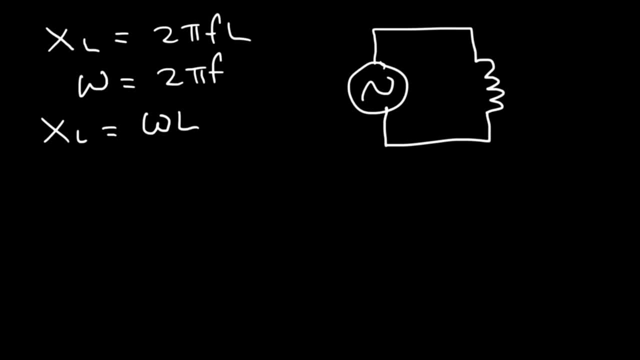 And as the current decreases, the energy stored in the inductor increases as well. So you can say that when the current Lifegov is dramatic enough as I can, you can see it here- the current in the inductor changes. But when you have an AC and the current of the 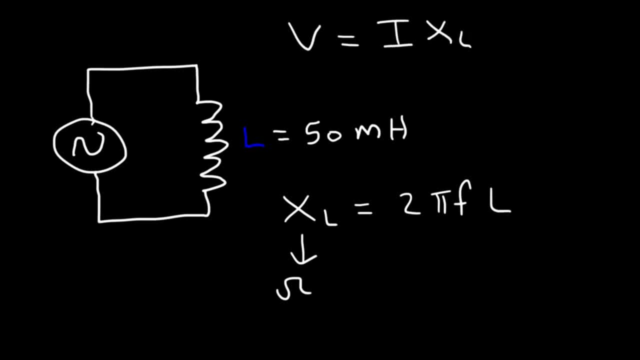 So, just as V equals IR, V is equal to I times xL. If you were to plot a graph between the frequency and the inductive reactance, these two are directly related. As the frequency increases, the inductive reactance increases as well. 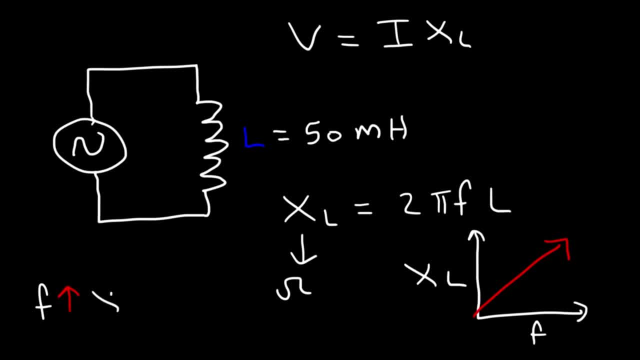 So when f goes up, xL goes up And as the inductive reactance goes up, the current in the circuit decreases. Current and inductive reactance are inversely related. So high frequency AC signals will yield less current in the circuit and low frequency 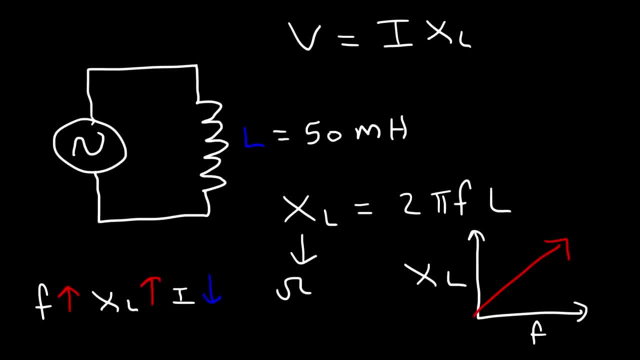 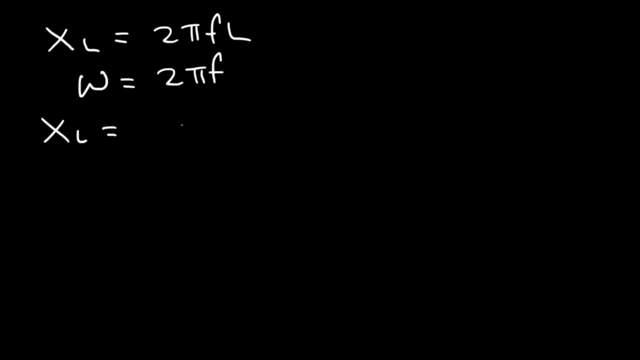 signals will yield less current. Now, going back to this equation where inductive reactance is equal to 2 pi fL, you need to know that omega, the angular frequency, is equal to 2 pi f, So xL can be represented as omega times L. So just keep that in mind. 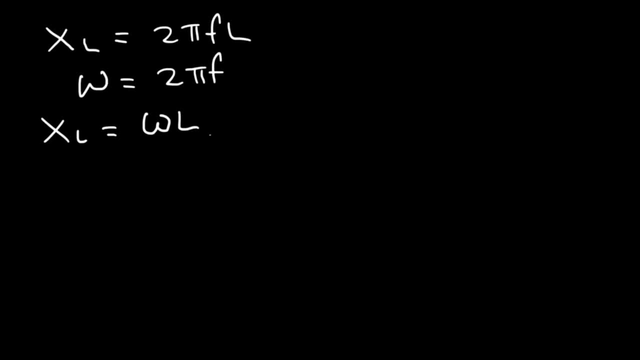 Also for an inductor, the current lags the voltage by 90. You need to know that as well. So that's it. Thanks for watching. See you next time. So whenever you have an AC signal passing through an inductor, the AC signal, the current. 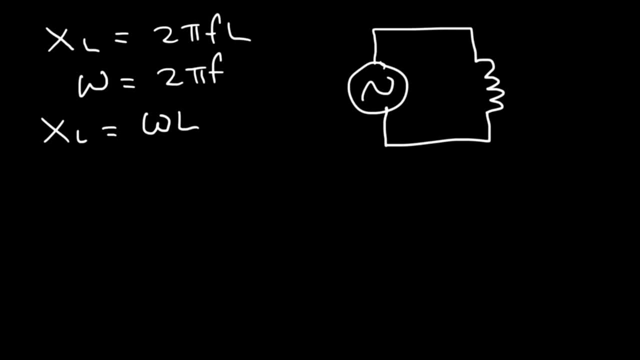 in. it is changing. It's increasing and decreasing. It's not constant And because the current changes you're going to have a change in magnetic flux inside the inductor. As the current increases, the energy stored in the inductor increases as well. 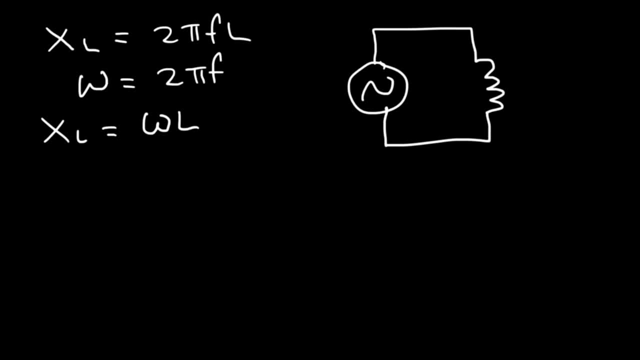 And as the current decreases, the energy stored in the inductor increases as well. The current in the circuit increases, so energy is stored in the inductor temporarily. The right side of this left receiver, this lovely, cool little business, and the right. one in the right receiver. it's in and around the nuquette. The inductor can move глазily era, tau, 007, or whatever, without the inductor, where energy is stored, so it can moveiteitus and it automatically moves laterach into the circuit. 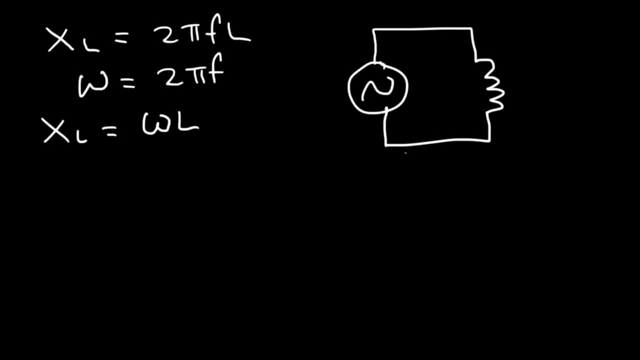 So energy is stored in the inductor temporarily. The inductor stores energy in the inductor in the indeftfer melee field and then it releases it back as the current in the circuit increases and decreases In can of the resistor, energy in the inductor is dissipated as heat. 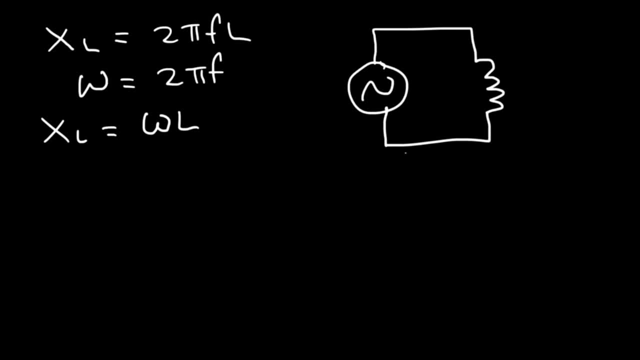 So that energy is gone. but in a case of an inductor, the energy is not gone. it is stored in the inductor temporarily, as heat energy is not gone. it is stored temporarily in the magnetic field of the inductor and 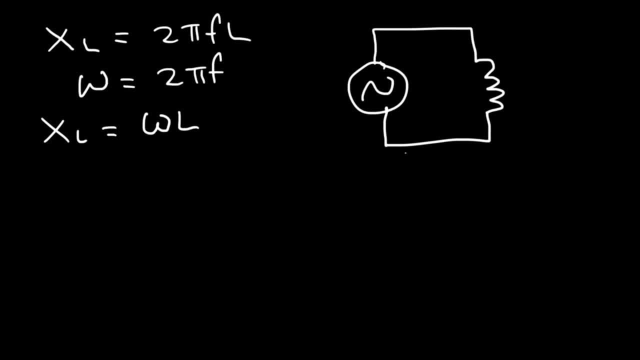 then it is released back to the source. Therefore, for all practical purposes, the inductor doesn't consume energy, it simply stores it and gives it back. So there's no loss in energy. Now, granted, no inductor is perfect. there's going to be some resistance in the coils of the 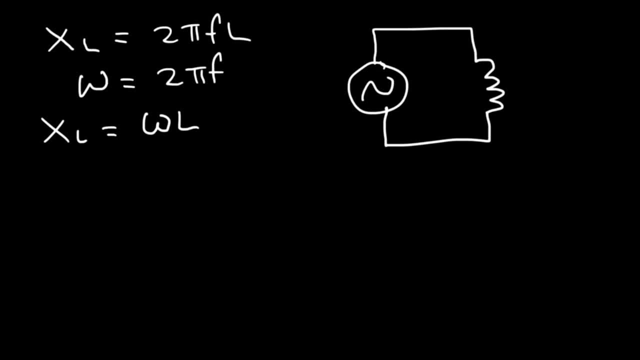 inductor and that resistance will dissipate energy as heat. But assuming if the inductor has no resistance, then it dissipates no energy, it simply stores it temporarily. Now let's talk about frequency. Let's say, if the frequency of the AC signal is 60 Hz, what 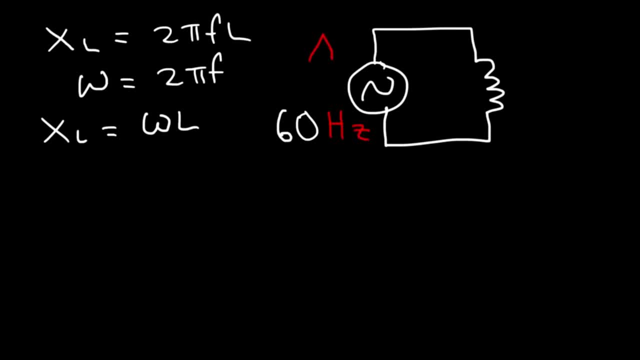 does that mean? This means that the alternating current changes direction 67 times in 1 second. Frequency is the number of cycles per second, so the current changes direction 60 times per second. Let's say, if the frequency changes direction 60 times in 1 second, the alternating current 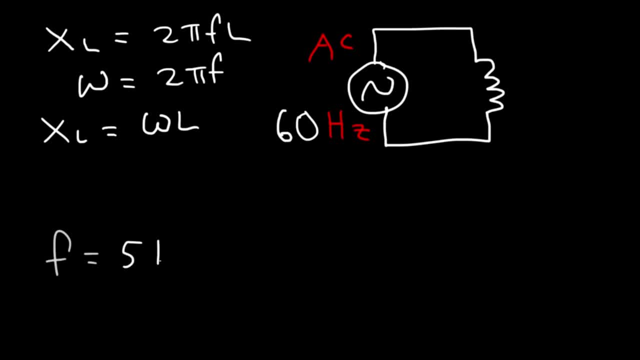 was 5 kilohertz. this is equal to 5,000 Hertz. that means that the AC signal changes direction 5,000 times in a single second. so whenever you see the word frequency in terms of an AC signal, that's what it means. now let's move on. 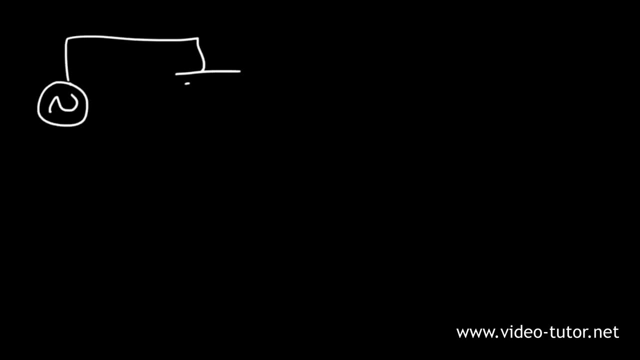 to a capacitive circuit. capacitive reactance is 1 over 2 PI F C and we know that Omega is 2 PI F. so capacitive reactance is 1 over Omega times C. so as the frequency increases, the capacitive reactance it decreases. notice that. 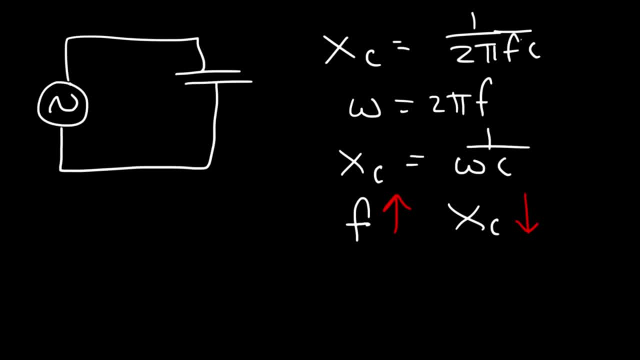 there's a little bit of a gap between the two capacitive reactants. so if you see the graph here, it's the same as the previous one, but the difference is F is on the bottom of the fraction, so F and X, C, the inversely related. if we were to 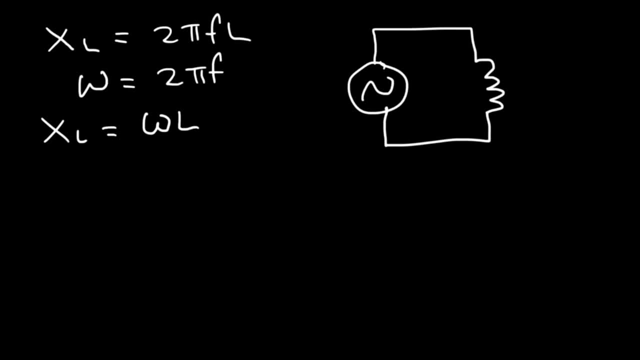 energy posture lose. favorably, It can be solved immediately. It says that the current in the inductor decreases, So energy is stored in the inductor temporarily. The inductor stores energy in this magnetic field and then releases it back as the current. 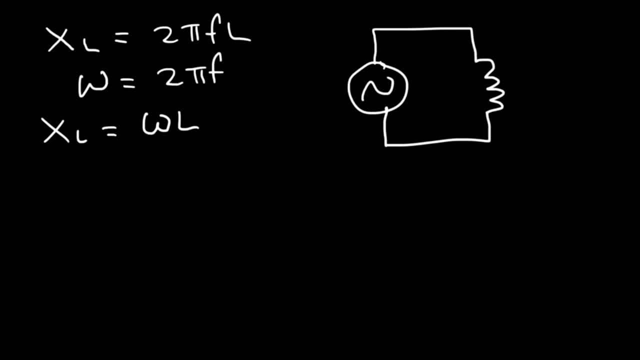 in the circuit increase and decreases. So in the case of a resistor, energy in the resistor is dissipated as heat, so that energy is gone in the inductor and then it is released back to the source. Therefore, for all practical purposes, 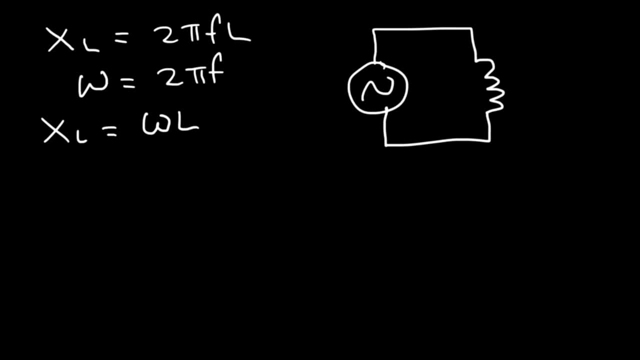 the inductor doesn't consume energy, It simply stores it and gives it back. So there's no loss in energy. Now, granted, no inductor is perfect. There's going to be some resistance in the coils of the inductor, and that resistance will dissipate energy as heat. But assuming if the 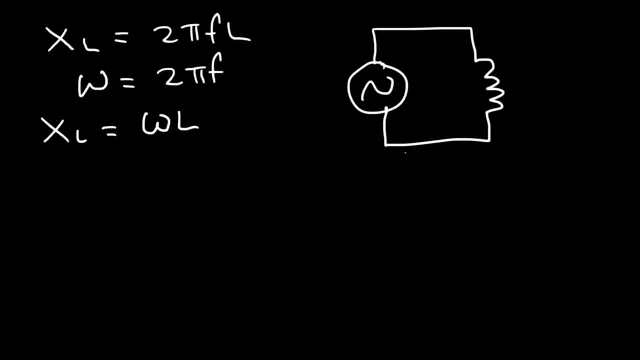 inductor has no resistance, then it dissipates no energy. It simply stores it temporarily. Now let's talk about frequency. Let's say, if the frequency of the AC signal is 60 hertz, What does that mean? This means that the alternating current changes direction 60 times. 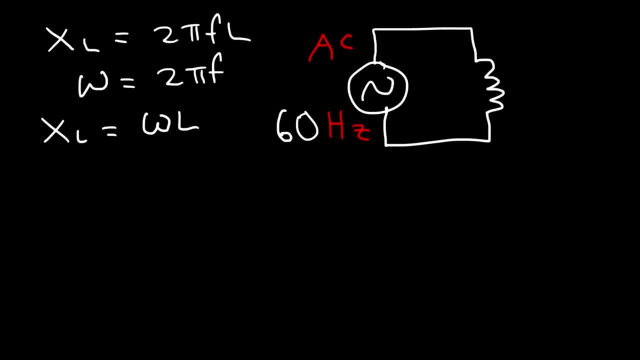 in one second. Frequency is the number of cycles per second. So the current changes direction 60 times per second. Let's say, if the frequency was 5 kilohertz, This is equal to 5,000 hertz. That means that the AC signal 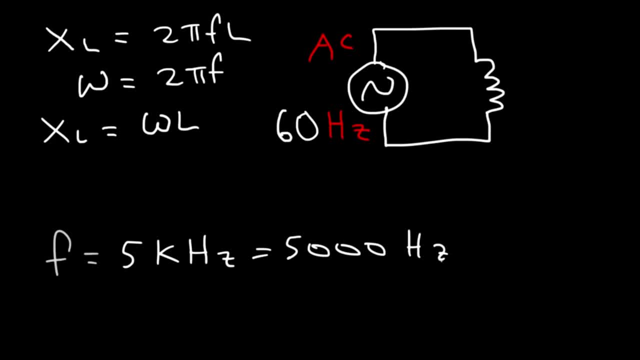 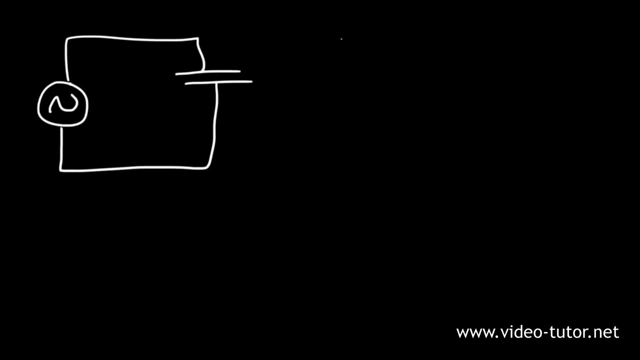 changes direction 5,000 times in a single second. So whenever you see the word frequency in terms of an AC signal, that's what it means. Now let's move on to a capacitive circuit. Capacitive reactants is 1 over 2 pi fc, And we know that omega is 2 pi f, So capacitive reactants is 1 over. 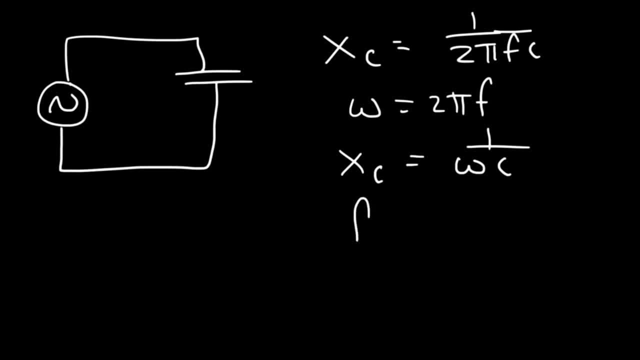 omega times c. So as the frequency increases, the capacitive reactants decreases. Notice that f is on the bottom of the fraction. So f and xc, they're both on the bottom of the fraction. So f and xc, they're inversely related. If we were to plot a graph between the capacitive reactants, 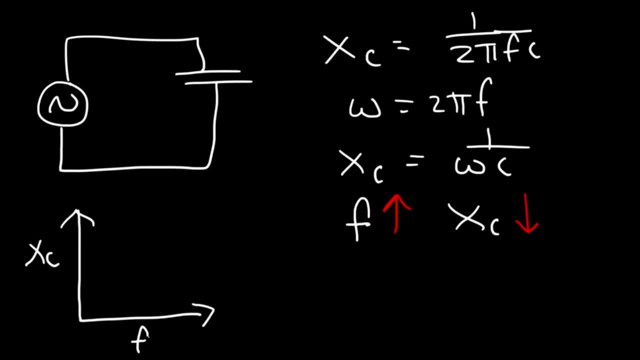 plot a graph between the capacitive reactance and a frequency. here's how it will look like: as the frequency goes up, the capacitive reactance goes down, so it's an inverse relationship, and the voltage in the circuit is equal to the current multiplied by the capacitive reactance. 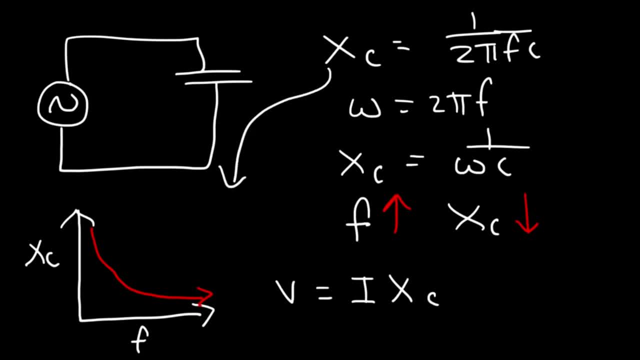 the capacitive reactance, like the inductive reactance and resistance, they all have the same unit and that is ohms, so just keep that in mind. by the way, for a capacitive circuit, and the current leads the voltage by 90, for an inductive, 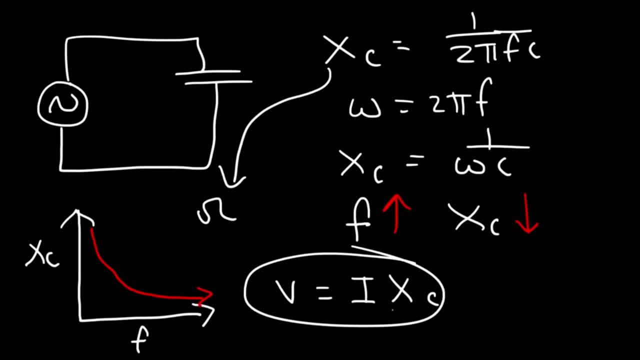 circuit lags the voltage by ninety. now, just as an inductor can store energy temporarily in its magnetic field, the capacitor energy will quickly vara dist 느ar from its magnetic field and the capacitor will not come offglich. Pacific fifth, that такой can store energy temporarily in its electric field. 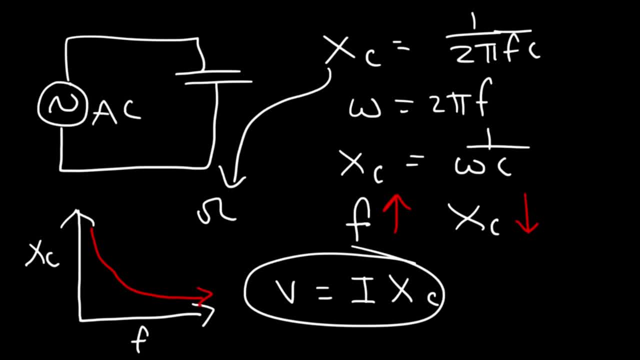 In an AC circuit, the voltage is constantly increasing and decreasing. It's basically a sine wave: The voltage goes up, then it goes down, and so forth. Whenever the voltage is increasing, the capacitor is storing energy, It's being charged. 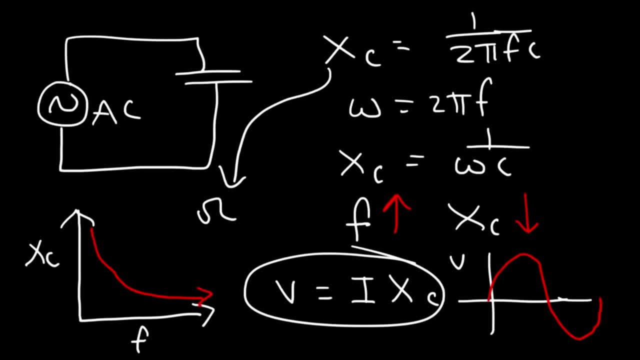 It's storing energy in its electric field And when the voltage decreases, the capacitor releases that stored energy, Because it absorbs and releases energy just like an inductor. the capacitor doesn't consume energy, So only the resistor consumes energy. It loses energy as heat. It doesn't give it back. 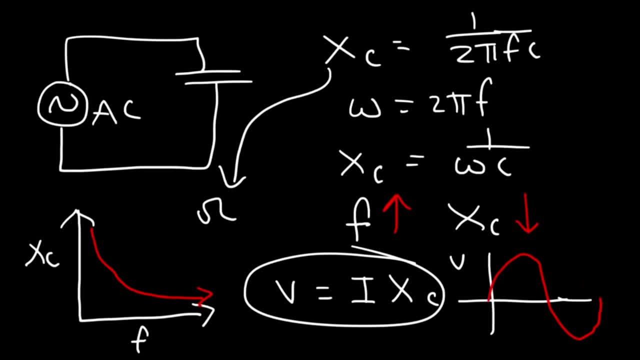 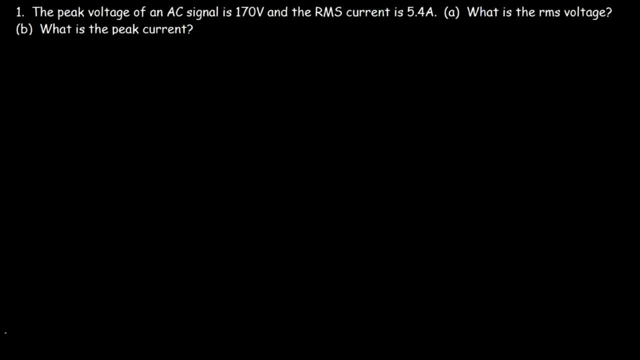 But capacitors and inductors. they store energy temporarily, So they dissipate no energy. Now let's work on some problems. Number one: The peak voltage of an AC signal is 170 volts and the RMS current is 5.4 amps. 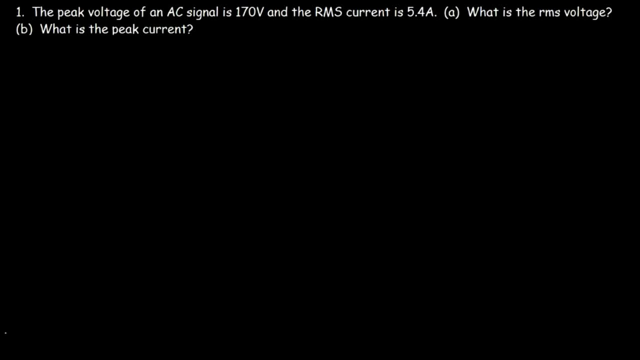 What is the RMS voltage? What is the peak current? To calculate the RMS voltage, it's simply equal to the peak voltage divided by the square root of 2.. The peak voltage is greater than the RMS voltage, and that's always going to be the case. 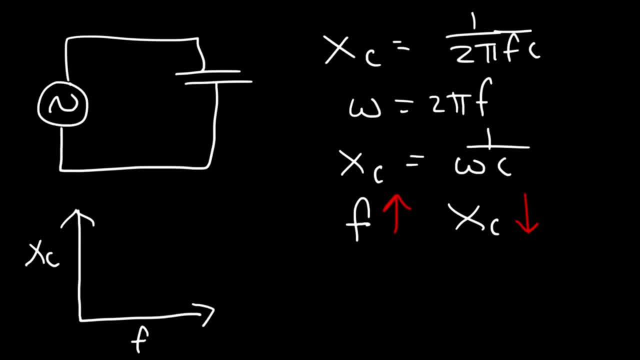 and the frequency. here's how it would look like: As the frequency goes up, the capacitive reactants goes down, So it's an inverse relationship And the voltage in the circuit is equal to the current multiplied by the capacitive reactants. The capacitive reactants, like the inductive, 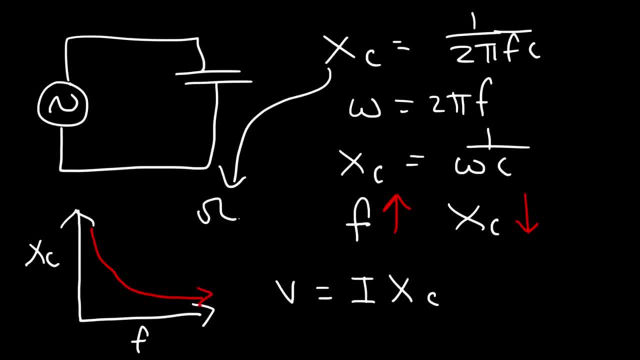 reactants and resistance. they all have the same unit and that is ohms. So just keep that in mind. By the way, for a capacitive circuit, the current leads the voltage by 90.. For an inductive circuit, the current lags the voltage by 90.. Now, just as an inductor can store energy temporarily in its 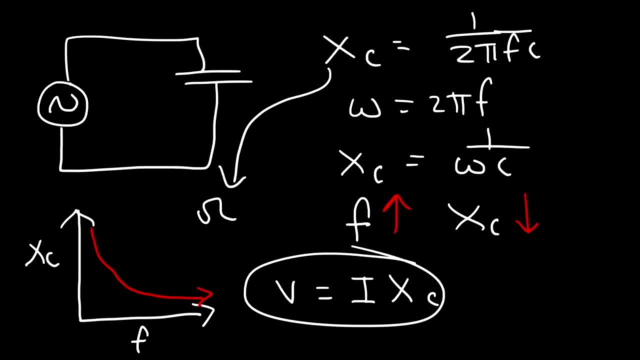 magnetic field, the capacitor can store energy temporarily in its electric field. In an AC circuit, the voltage is constantly increasing and decreasing. It's basically a sine wave: The voltage goes up, then it goes down, and so forth. Whenever the voltage is increasing, the capacitor is storing energy, It's being charged. 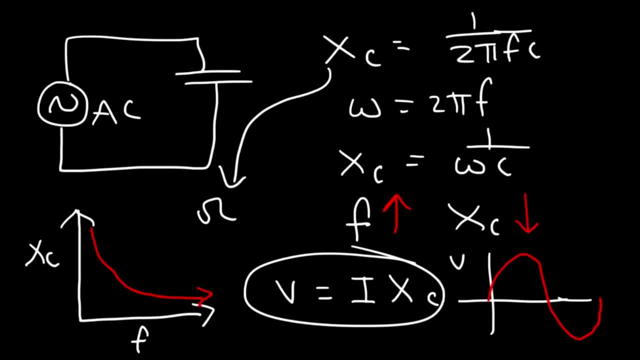 It's storing energy in its electric field And when the voltage decreases the capacitor releases that stored energy. Because it absorbs energy. the capacitor is going to start doing Theo-Kakes' Norwegian value, then releases energy, just like an inductor. the capacitor doesn't consume energy, So only the 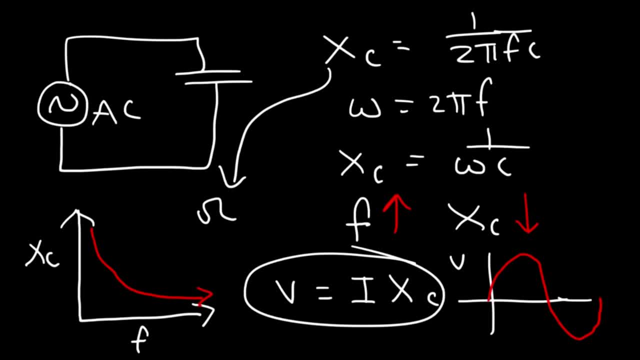 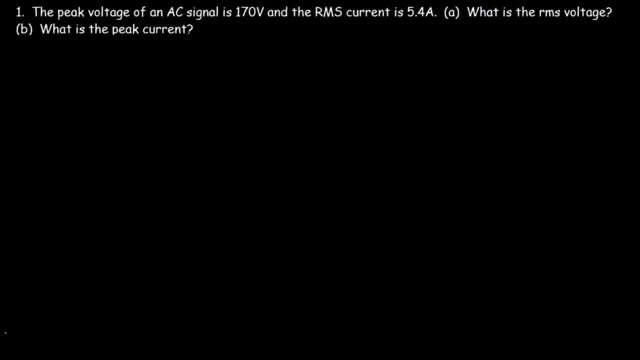 resistor consumes energy. It loses energy as heat, It doesn't give it back. But capacitors and inductors: they store energy temporarily, So they dissipate no energy. Now let's work on some problems. Number one: the peak voltage of an AC signal is 170 volts and the RMS current is 5.4. 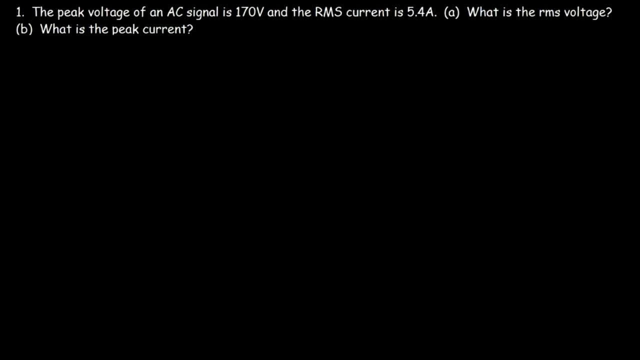 amps. What is the RMS voltage? What is the peak current? To calculate the RMS voltage, it's simply equal to the peak voltage divided by the square root of 2.. The peak voltage is greater than the RMS voltage, and that's always going to be the case. So it's 170 volts divided by root 2.. 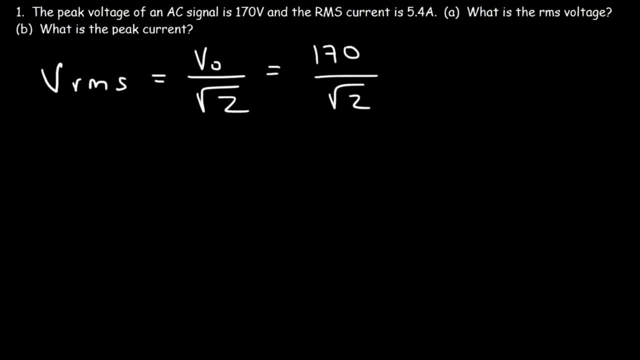 So it's 170 volts Divided by root 2.. So this is equal to 120.2 volts. Now part B: What is the peak current? The RMS current is equal to the peak current divided by the square root of 2.. 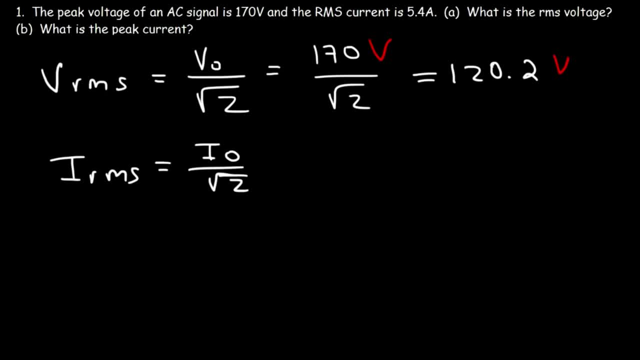 So if we rearrange the equation by multiplying both sides by root 2, the peak current is equal to the RMS current times root 2.. So it's going to be the square root of 2 times 5.4 amps. So this is going to be about 7.64 amps. 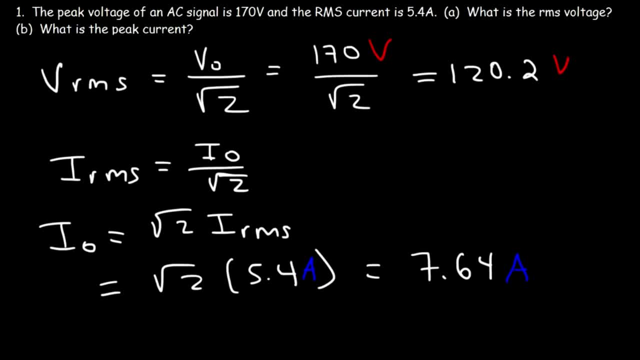 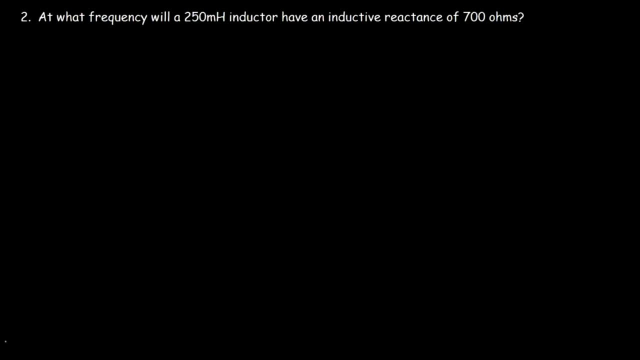 So the peak current is 0.8.. So the peak current is always greater than the RMS current And the RMS voltage, or the RMS current, is always less than the peak value Number 2.. At what frequency will a 250 milliHenry inductor have an inductive reactance of 700 ohms? 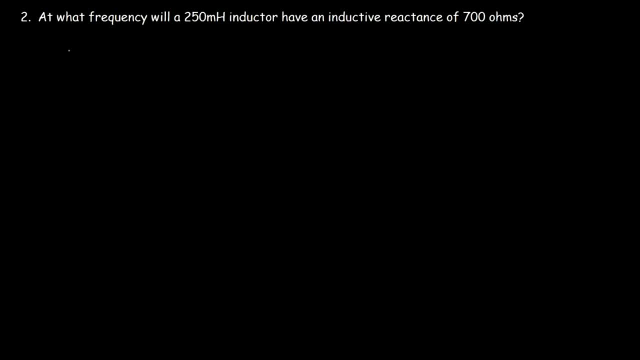 So feel free to try this problem. The inductive reactance is equal to 2 pi times the frequency times the inductance. The inductive reactance has unit ohms, so it's 700 ohms. We're looking for F, the frequency. 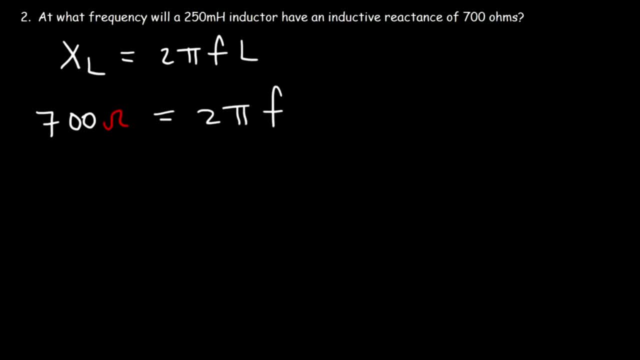 And L is the inductance of the inductor, which is measured in henries, or in this case milliHenries. So 250 milliHenries is basically 0.25 Henries. You've got to divide it by 1,000 to convert milliHenries to Henries. 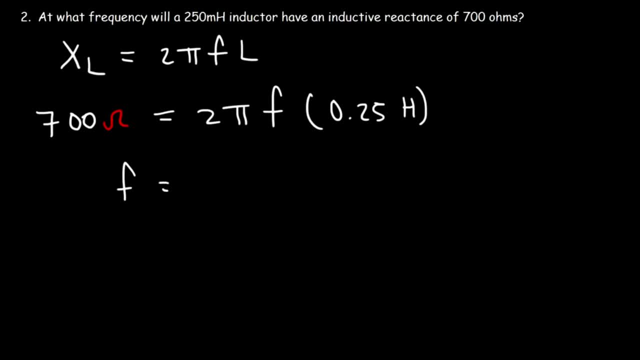 So the frequency? The frequency is going to be 700 divided by 2 pi times 0.25.. So it's going to be about 445.6 Hertz. This frequency will produce an inductive reactance of 700 ohms. 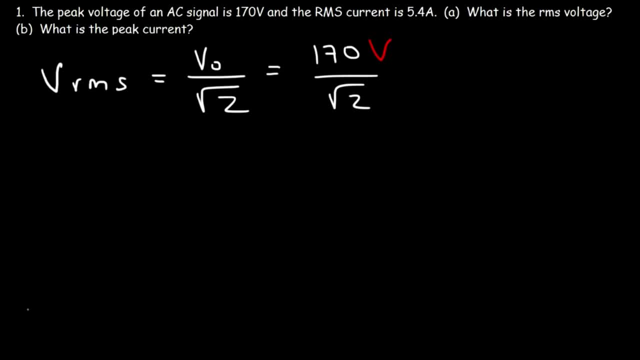 So this is equal to 120.2 volts. Now part B: what is the peak current? The RMS current is equal to the peak current divided by the square root of 2.. So if we rearrange the equation by multiplying both sides by root 2, the peak current is equal to the RMS current times root 2.. 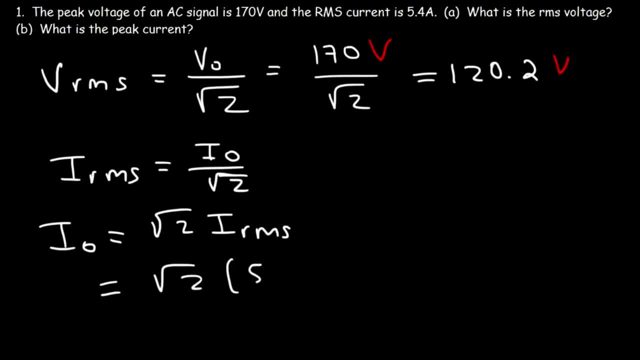 So it's going to be the square root of 2 times 5.4 amps. So this is going to be about 7.64 amps. So the peak current is always greater than the RMS current And the RMS voltage, or the RMS. 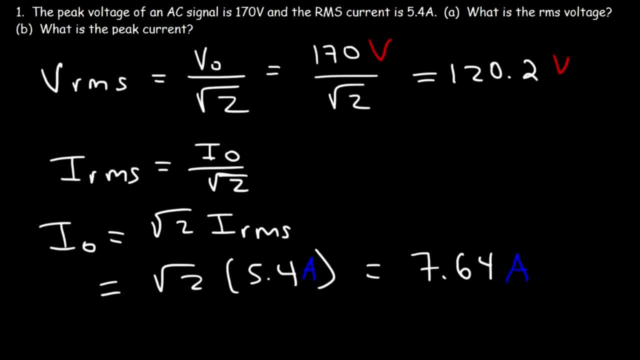 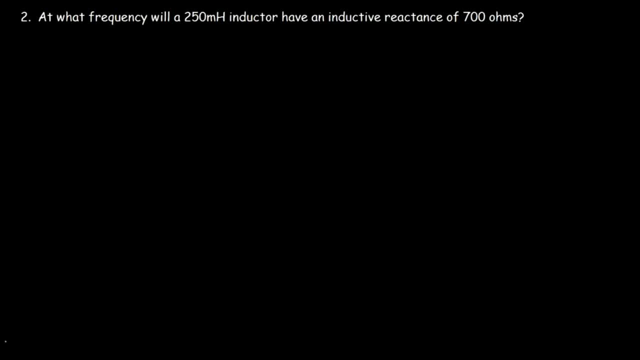 current is equal to the peak current. So the peak current is always greater than the RMS current. So the peak current is always greater than the RMS current. So the peak current is always less than the peak value. Number two: at what frequency will a 250 milliHenry inductor have an inductive reactance of 700? 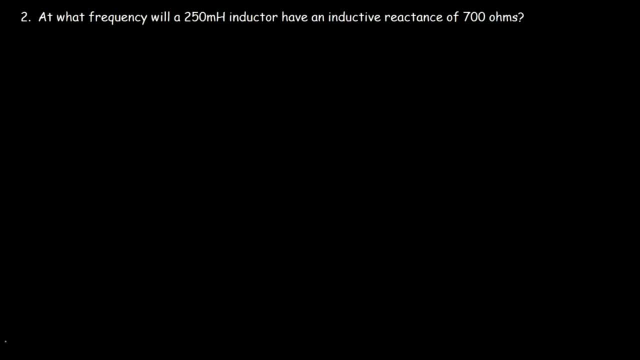 ohms, So feel free to try this problem. The inductive reactance is equal to 2 pi times the frequency, times the inductance. The inductive reactance has unit ohms, so it's 700 ohms. We're looking for F, the frequency, And L is the inductance of the inductor, which is 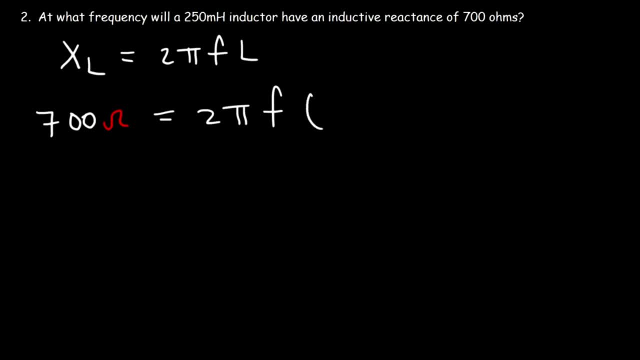 measured in Henrys, or in this case in milliHenrys. So 250 milliHenrys is basically 0.25 Henrys. You got to divide it by 1,000 to convert milliHenrys to Henrys. So the frequency is going to be: 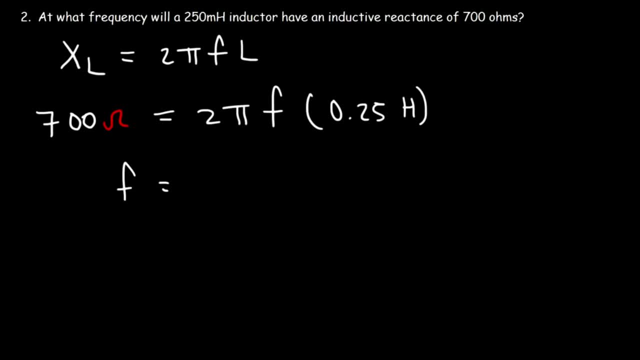 700 divided by 2 pi times 0.25.. So it's going to be about 445.6 Hertz. This frequency will produce an inductive reactance of 700 ohms. Number three: a 60 Hertz AC signal at 120 volts is connected across a 500 milliHenry. 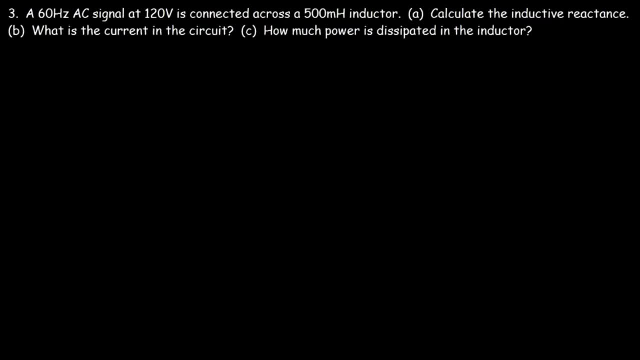 Number 3.. A 60 Hertz AC signal at 120 volts is connected across a 500 milliHenry inductor. Calculate the inductive reactance. So let's begin by drawing a picture. So here's the AC signal And here is the inductor. 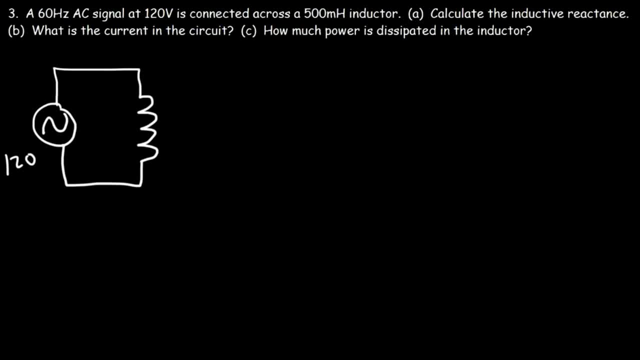 So the voltage is 120.. And the frequency is 60 Hertz And the inductance is 500 milliHenries. So to find the inductive reactance let's use this equation: It's 2 pi times F times L. 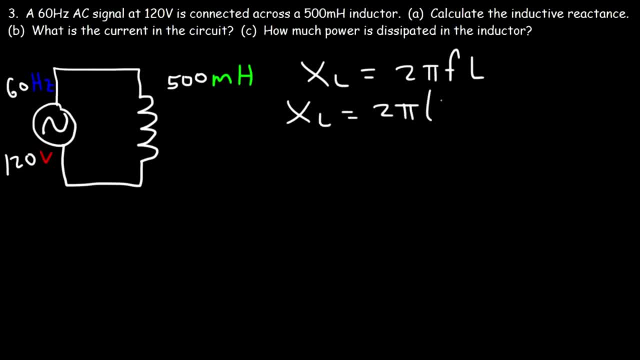 So the frequency is 60. And L 500 milliHenries. that's the same as 0.5 Henries if you divide it by 1,000.. So 60 times 0.5 is 30 times 2 pi. 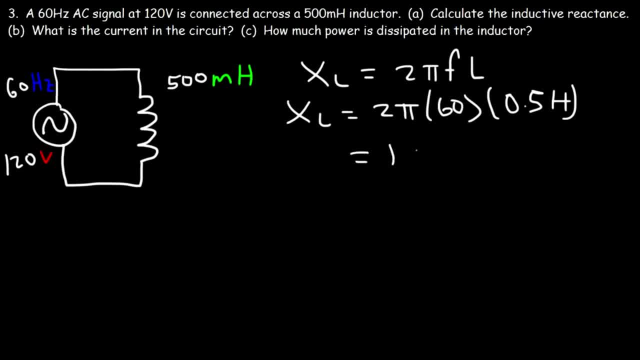 That's 60 pi, which is 188.5.. So that's the inductive reactance. Once we have that, we can find the current in the circuit. So V is equal to I times XL, Which means that the current is equal to the voltage divided by the inductive reactance. 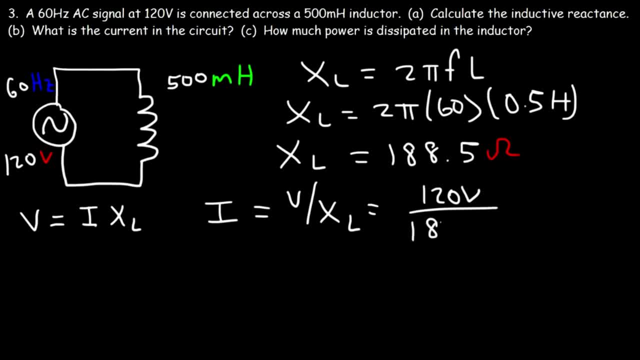 The voltage is 120.. And the inductive reactance is 188.5.. So the current in the circuit is 0.6366 amps. Now what about part C? How much power is dissipated in the inductor? The inductor doesn't dissipate anything. 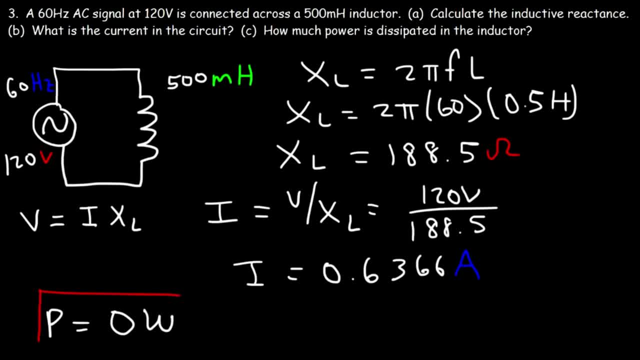 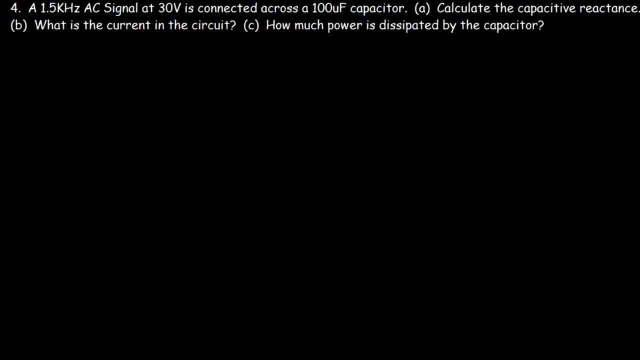 So it's 0 watts. It simply stores energy temporarily in its magnetic field And then it releases it back. And it's constantly doing it. It's constantly absorbing energy and releasing energy, So it doesn't consume energy. Note Number four: a 1.5 kilohertz AC signal at 30 volts is connected across a 100 microfarad capacitor. 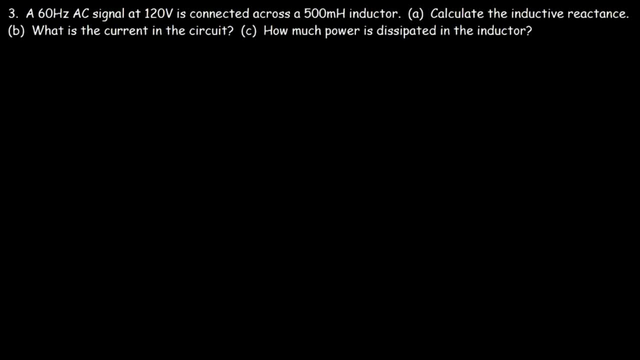 inductor, Calculate the inductive reactance. So let's begin by drawing a picture. So here's the AC signal and here is the inductor. So the voltage is 120, and the frequency is 60 Hertz And the inductance is 500 milliHenrys. So to find the inductive reactance, let's use 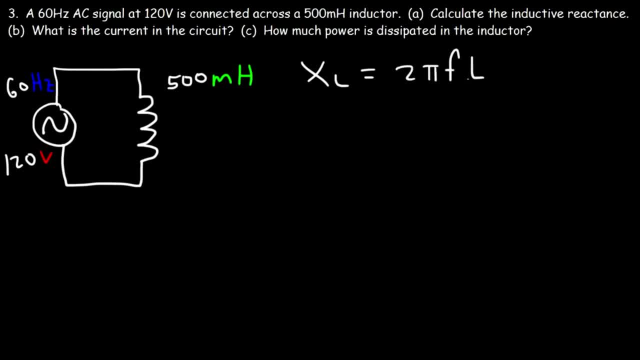 this equation: It's 2 pi times F times L, So the frequency is 60, and L 500 milliHenrys. that's the same as 0.5 Henrys if you divide it by 1,000.. So 60 times 0.5 is 30, times 2 pi. That's 60 pi, which is 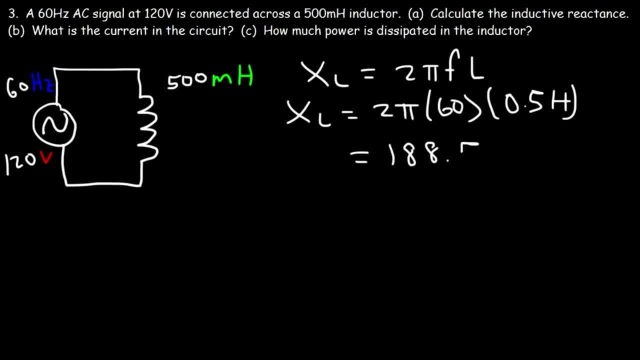 188.5 ohms. So that's the inductive reactance. Once we have the inductive reactance, we're going to be able to calculate the inductive reactance. If we have that, we can find the current in the circuit. So V is equal to I times XL. 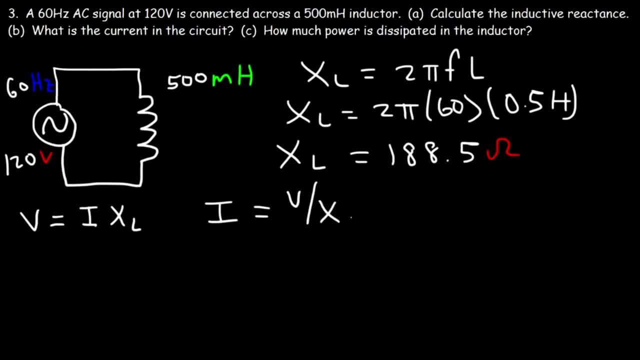 which means that the current is equal to the voltage divided by the inductive reactance. The voltage is 120, and the inductive reactance is 188.5.. So the current in the circuit is 0.6366 amps. Now what about part C? How much power is dissipated in the inductor? The inductor doesn't dissipate. 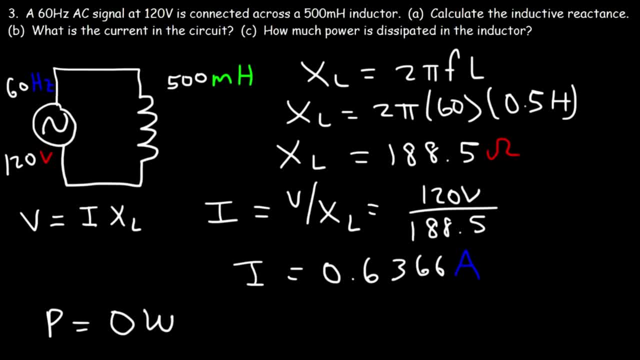 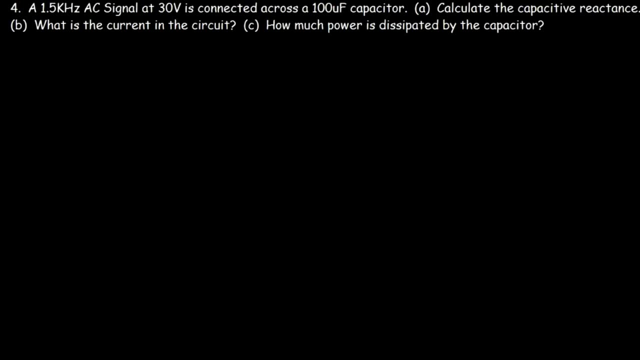 anything. So it's zero watts. It simply stores energy temporarily in its magnetic field and then it releases it back. And it's constantly doing it. It's constantly absorbing energy and releasing energy, So it doesn't consume energy. Number four: a 1.5 kilohertz AC signal at 30. 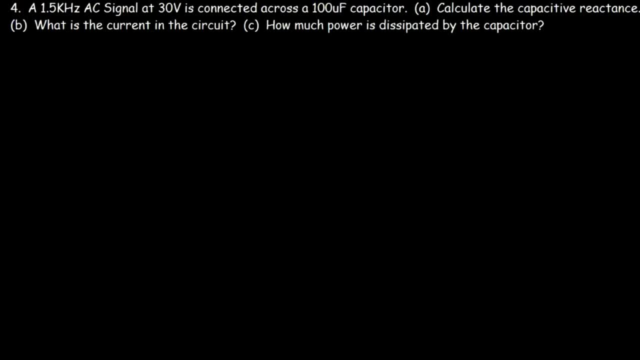 volts is connected across the circuit, So it's 0.5 kilohertz AC signal at 30 volts, So it's connected across a 100 microfarad capacitor. Calculate the capacitive reactance. So here is the AC signal and it's directly across a capacitor, So the signal is at 30 volts. 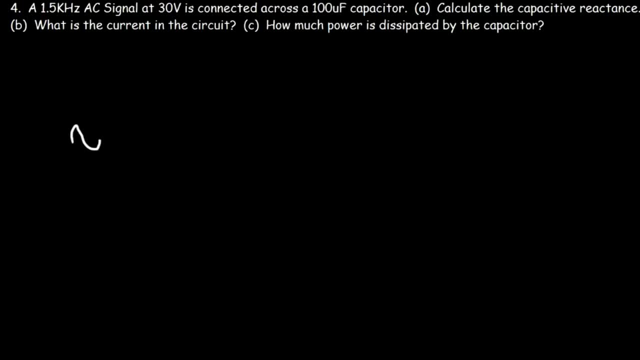 Calculate the capacitive reactance. So here is the AC signal and it's directly across a capacitor, So the signal is at 30 volts and 1.5 kilohertz And the capacitance Is 100 microfarads. So let's begin by calculating the capacitive reactance, which is Xc. 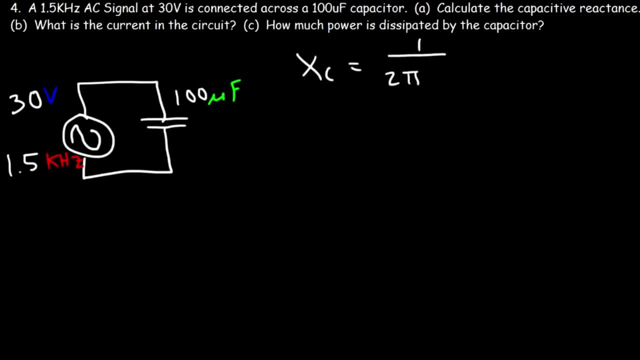 And it's equal to 1 divided by 2 pi Fc. So it's 1 over 2 pi times the frequency. 1.5 kilohertz is 1500 hertz. You got to multiply it by 1000 to convert it to hertz. 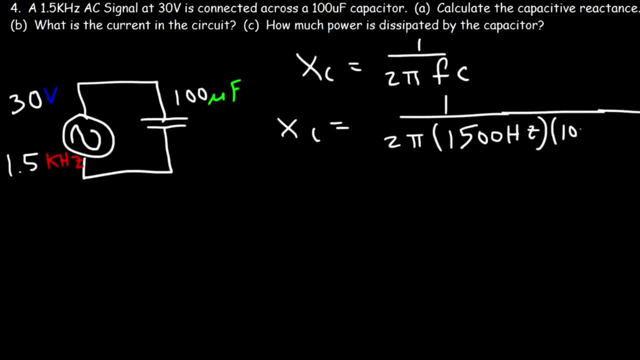 And 100 microfarads is basically 100 times 10 to the minus 6 farads. So anytime you hear the word kilo it's 10 to the 3 mega, 10 to the 6 milli, 10 to minus 3 micro at 10 to negative 6.. 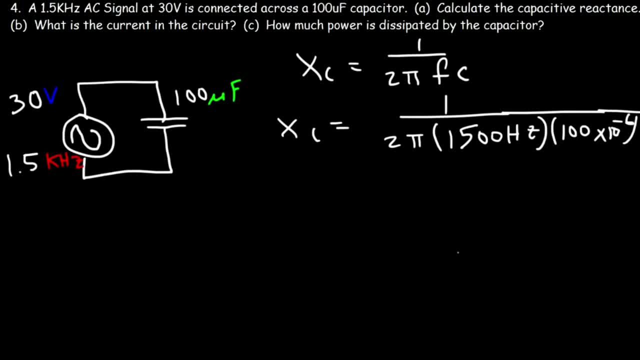 So if we multiply 2 pi times 1500 times 100, times 10 to minus 6. You should get 0.9425, and 1 divided by that number Is 1.061.. So this is the capacitive reactance of the circuit. 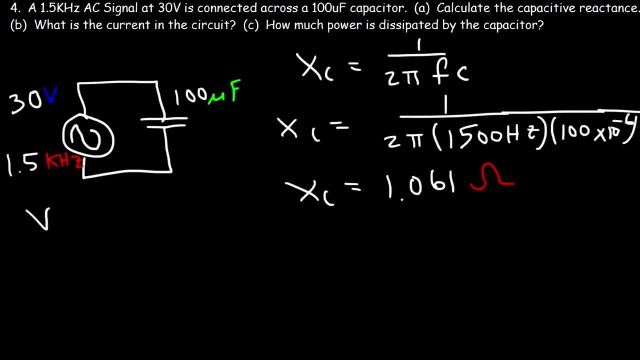 Now what is the current in the circuit? So V is equal to I times Xc, which means I is V over Xc. So it's 30 volts divided by 1.0.. So this yields a current of 28.3 amps. 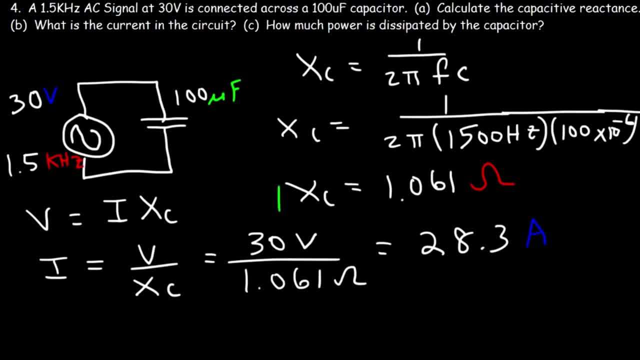 So that's the answer to part B. Now part C: how much power is dissipated by the capacitor? Like the inductor, the capacitor doesn't dissipate anything, So it's 0 watts. It stores energy in its electric field. 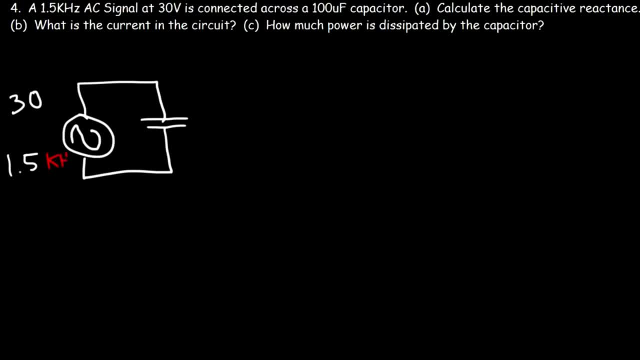 and 1.5 kilohertz And the capacitance is 100 microfarads, So it's directly across a capacitor. So let's begin by calculating the capacitor reactance, which is XC, and it's equal to 1 divided by 2 pi FC, So it's 1 over 2 pi times the frequency. 1.5 kilohertz is 1,500 hertz. 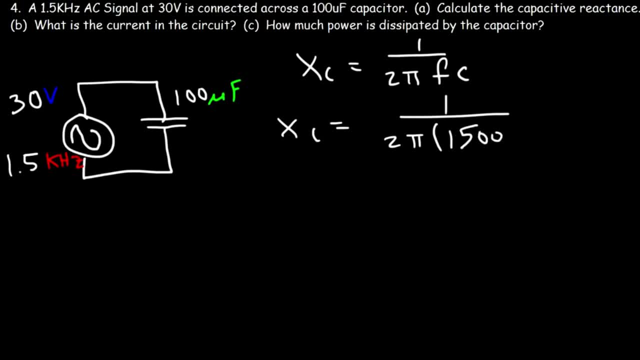 You got to multiply it by 1,000 to convert it to hertz, And 100 microfarads is basically 100 times 10 to the minus 6 farads. So any time you hear the word kilo, it's 10 to the 3. Mega. 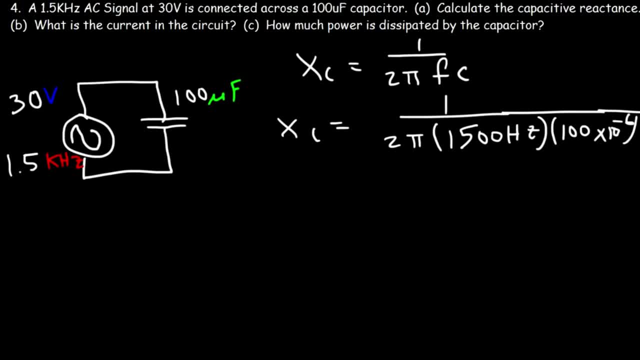 10 to the 6. Milli, 10 to the minus 3. Micro, add 10 to the negative 6. So if we multiply 2 pi times 1,500 times 100 times 10 to the minus 6,, 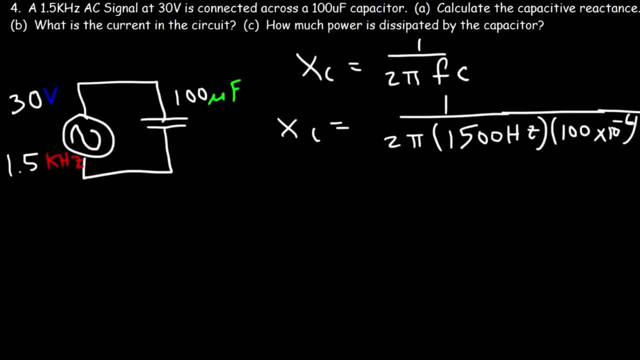 you should get 0.9425.. Divided by that number is 1.061.. So this is the capacitive reactance of the circuit. Now what is the current in the circuit? So V is equal to I times XC, which means I is V over XC. 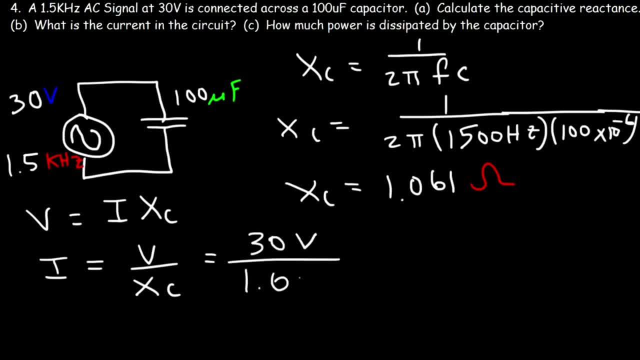 So it's 30 volts divided by 1.061 ohms. So this yields a current of 28.3 amps. So that's the answer to part B. Now part C: how much power is dissipated by the capacitor? 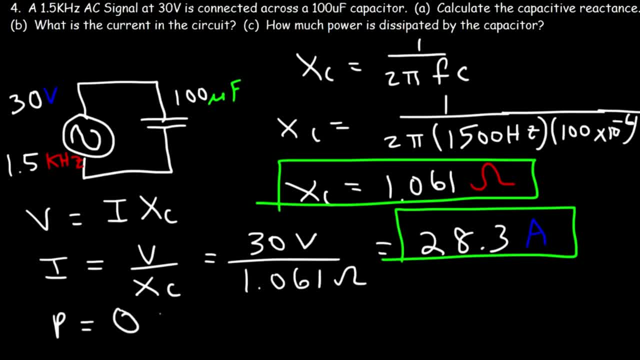 Like the inductor, the capacitor doesn't dissipate anything, So it's zero watts. It stores energy in its electric field and then temporarily releases it back. So this is the answer to part C. For those of you who want to access the circuit, you can do that by clicking the button on the right side of the screen. 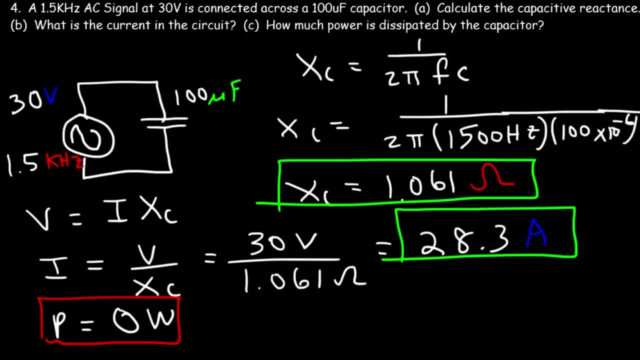 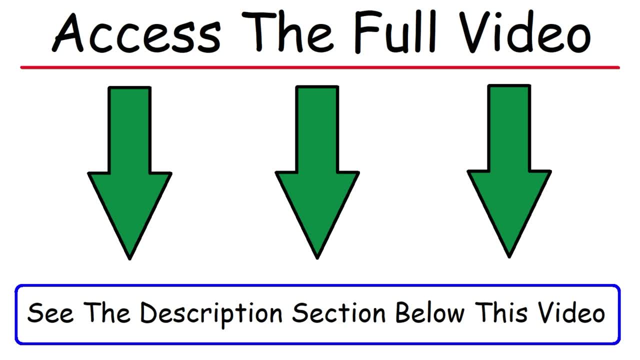 And then It temporarily releases it back. So this is the answer to part C. For those of you who want to access the full length version of this video, See the links in the description section below this video. You can access it on my Patreon page, patreoncom slash math science tutor. 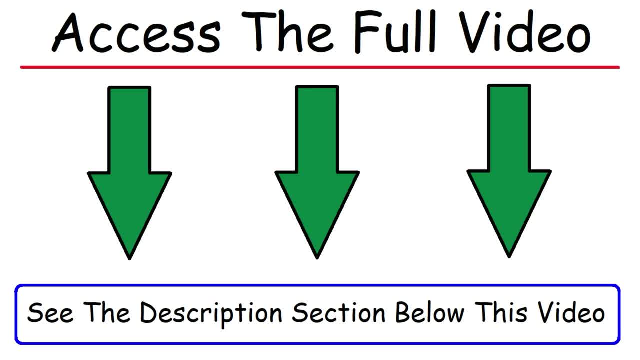 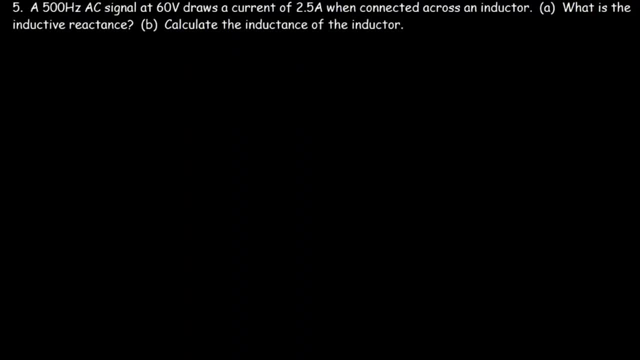 Or you can join my YouTube channel membership program to get those videos as well. So feel free to take a look. I'll look at that when you get a chance. Number five: a 500 hertz AC signal at 60 volts draws a current of 2.5 amps when connected across an inductor. 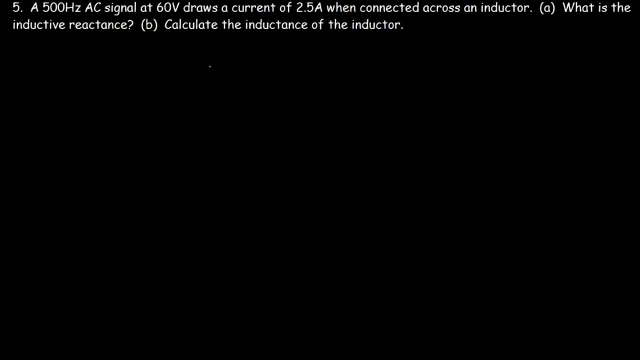 What is the inductive reactance? So let's make a list of what we have. We know the frequency is 500 hertz And we have the voltage. The voltage is 60 volts. And we also know the current, Which is 2.5 amps. 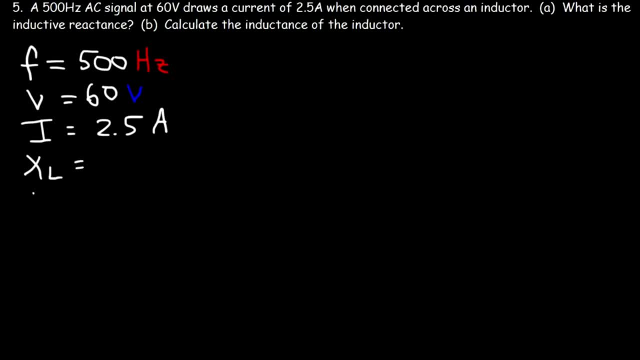 So what we're looking for is the inductive reactance and also the inductance. Well, we know that V is equal to I times XL, So XL is the voltage divided by the current 60 volts, divided by 2.5 amps. 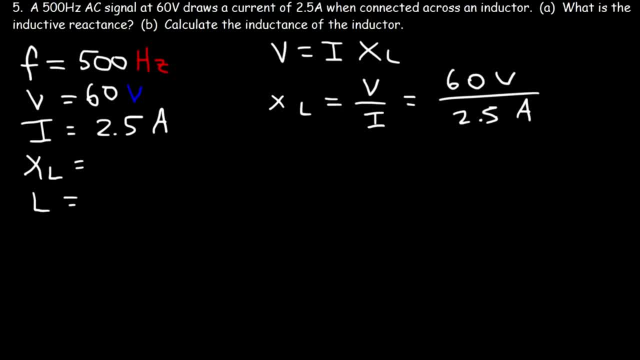 So 60 divided by 2.5.. That gives us an inductance or an inductive reactance rather of 24 ohms. So that's the answer to part A. Part B: what is the inductance? 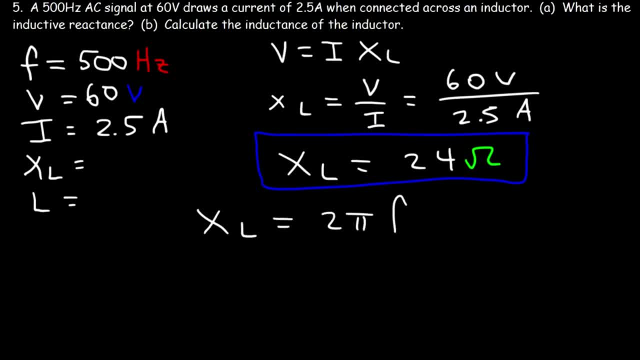 So once we have XL, we can use this equation to find L. So 24 is equal to 2 pi times the frequency of 500 times L. 2 pi times 500 is 1000 pi, So L is going to be 24 divided by 1000 pi. 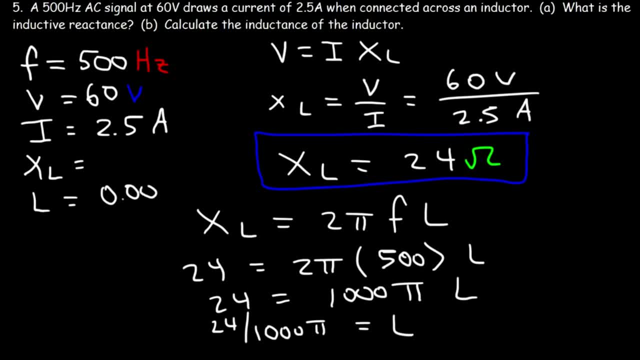 And so L is 0.00764 henries. To convert that to millihenries, multiply by 1000.. So it's about 7.64 millihenries. So that's the inductance. Now there are some other circuits that you need to be familiar with. 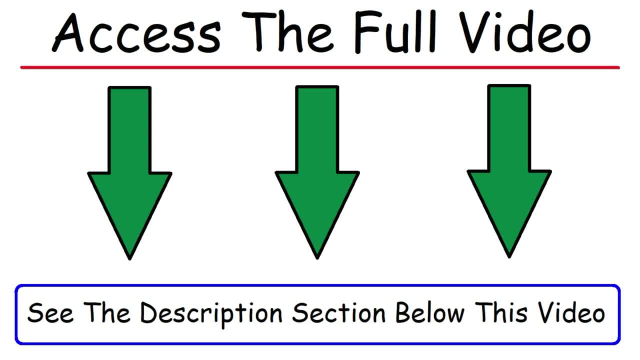 To access the full length version of this video, see the links in the description section below. this video You can access it on my Patreon page, patreoncom slash mathsciencetutor, Or you can join my YouTube channel membership program to get those videos as well. 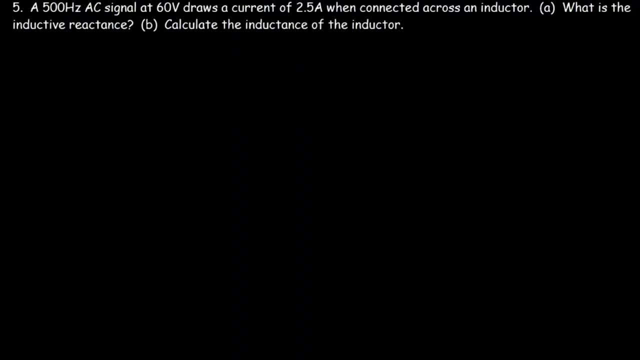 So feel free to take a look at that when you get a chance. Number five: a 500-hertz AC signal at 60 volts draws a current of 2.5 amps when connected across an inductor. What is the inductive reactance? 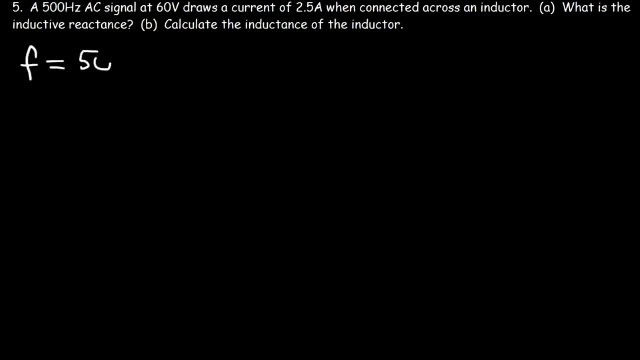 So let's make a list of what we have. We know the frequency is 500 hertz And we have the voltage- The voltage is 60 volts. And we also know the current, which is 2.5 amps. So what we're looking for is: 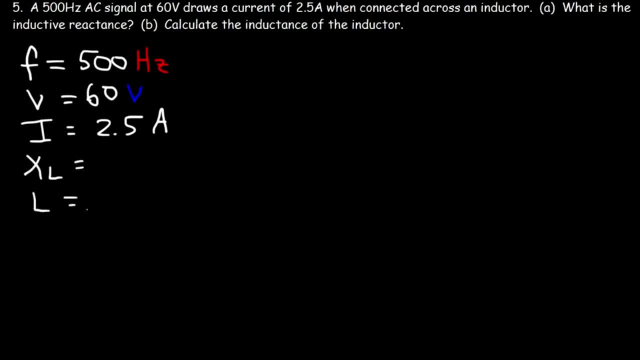 the inductive reactance and also the inductance. Well, we know that V is equal to I times XL. So XL is the voltage divided by the current 60 volts divided by 2.5 amps. So 60 divided by 2.5. 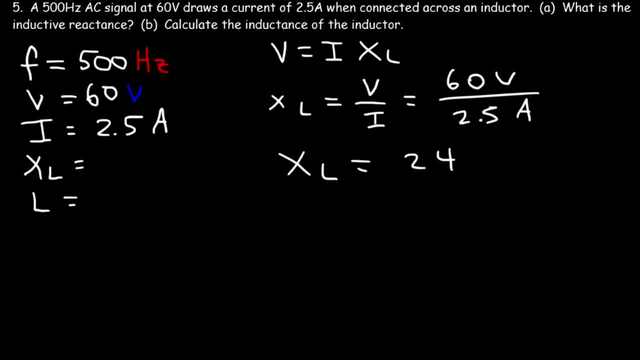 That gives us an inductance Or an inductive reactance Rather of 24 ohms. So that's the answer to part A. Part B: what is the inductance? So once we have XL, we can use this equation to find L. 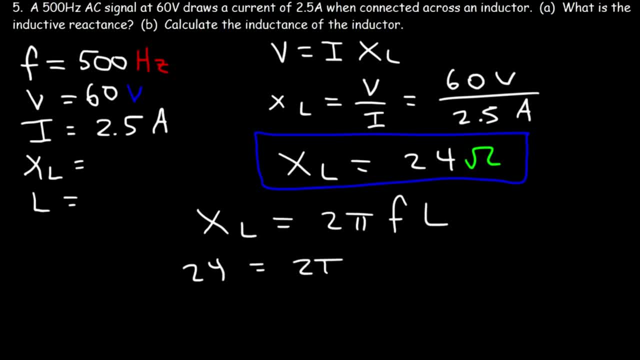 So 24 is equal to 2 pi times the frequency of 500 times L. 2 pi times 500 is 1,000 pi. So L is going to be 24 divided by 1,000 pi, And so L is 0.00764 henrys. 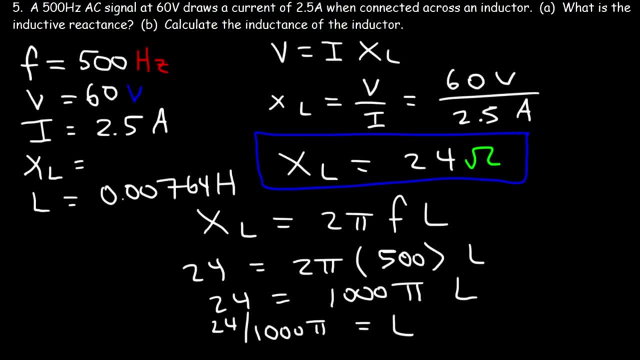 To convert that to millihenrys, multiply by 1,000.. So it's about 7.64 millihenrys. So that's the inductance. Now there are some other circuits that you need to be familiar with. 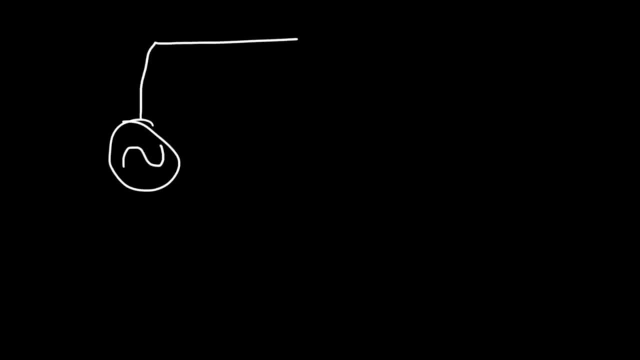 Let's talk about three different types. One circuit contains a resistor, an inductor and also a capacitor, So this circuit is known as an RLC circuit, because it has all three elements. The other two looks like this. So on the left we have a resistor and a capacitor. 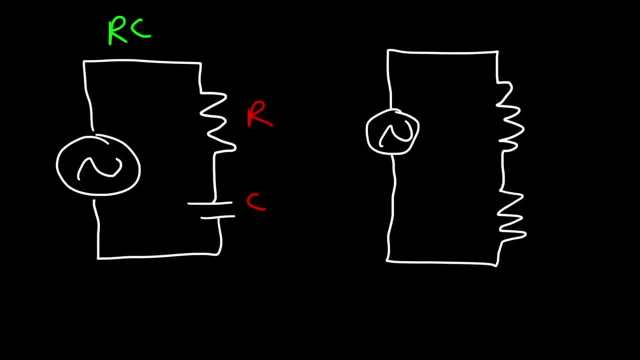 So that's known as an RC circuit. On the right we have a resistor and an inductor, So it's known as an RL circuit. For each of these circuits, Z, which is the impedance, is equal to the square root of R squared plus XL, minus XC squared. 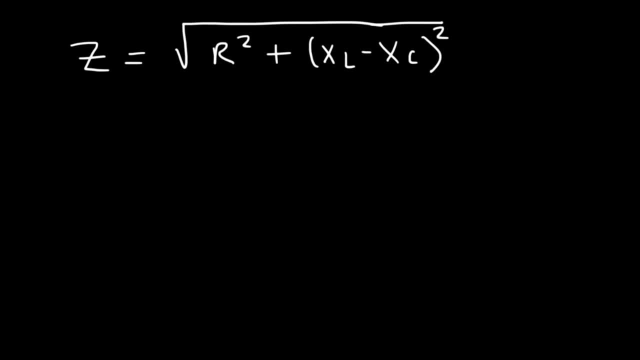 So for an RLC circuit, that's the equation that you're going to have. For an RL circuit, there is no XC, XC is 0, so it's just going to be R squared plus XL squared. And for an RC circuit, there is no XL. 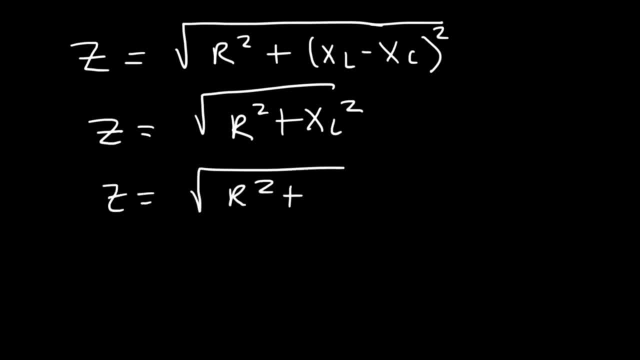 Z is going to be R squared, So it's going to be R squared plus XC squared. Now let's go back to the RLC circuit. The voltage across the resistor is known as Vr, And this is equal to the current multiplied by the resistance. 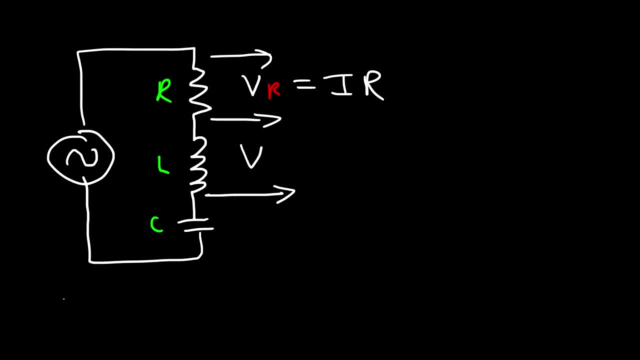 The voltage across the inductor. this is known as Vl And it's equal to the current times, the inductive reactance. And the voltage across the capacitor, Vc. that's going to be equal to the current in the circuit times, the capacitive reactance. 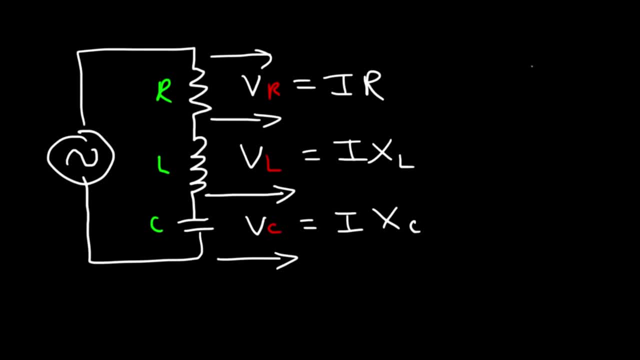 Now, if you want to find the current that flows in the circuit, the current is going to be equal to the current in the circuit. The current is going to be the voltage divided by the impedance. Z. R is the resistance in ohms. 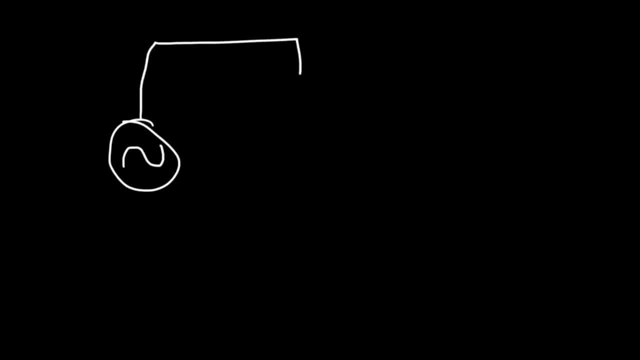 Let's talk about three different types. One circuit contains a resistor, an inductor and also a capacitor. So this circuit is known as an RLC circuit, because it has all three elements. The other two. It looks like this: So on the left we have a resistor and a capacitor. 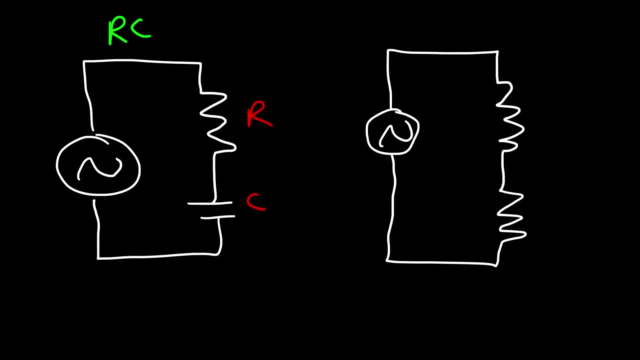 So that's known as an RC circuit. On the right we have a resistor and an inductor, So it's known as an RL circuit. For each of these circuits, Z, which is the impedance, is equal to the square root of R squared plus XL, minus XC squared. 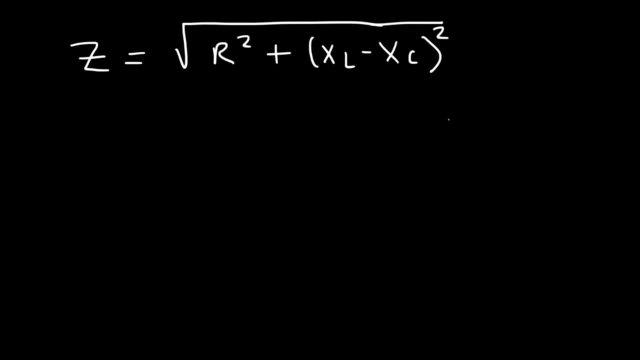 So for an RLC circuit, that's the equation that you're going to have. For an RL circuit, there is no XC, XC is 0, so it's just going to be R squared plus XL squared. And for an RC circuit, there is no XL. 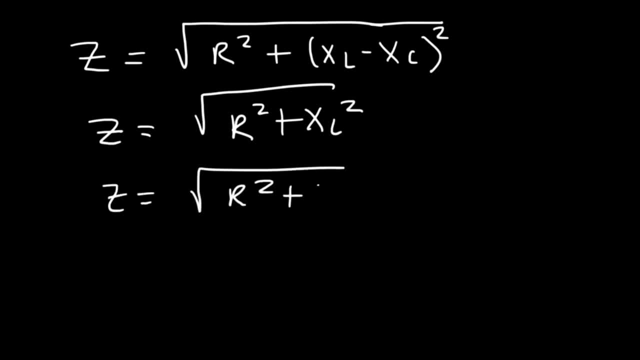 Z is going to be R squared plus XC squared. Now let's go back to the RLC circuit. The voltage across the resistor is known as VR, And this is equal to the current multiplied by The voltage across the inductor. this is known as VL. 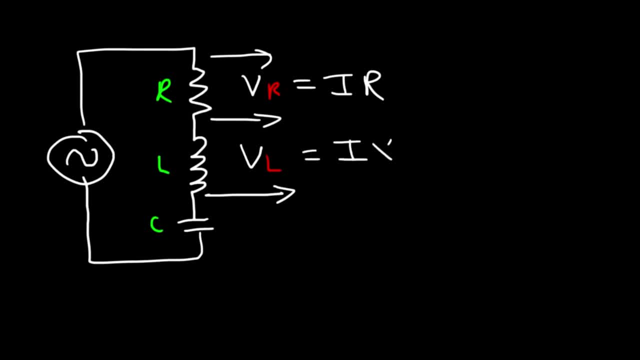 And it's equal to the current times, the inductive reactance, And the voltage across the capacitor VC. that's going to be equal to the current in the circuit times, the capacitive reactance. Now, if you want to find the current that flows in the circuit, 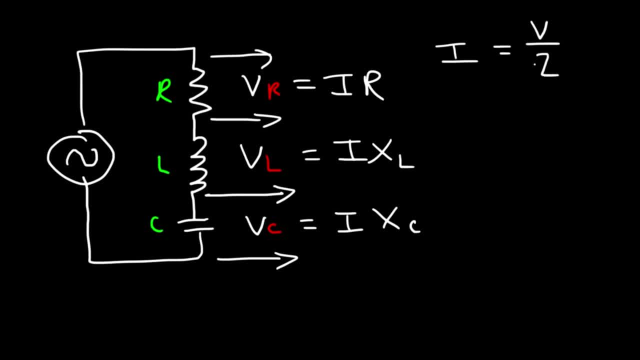 the current is going to be the voltage divided by the impedance. Z. R is the resistance in ohms. XL is the inductive reactance, which is also in ohms XC. the capacitive reactance is in ohms. 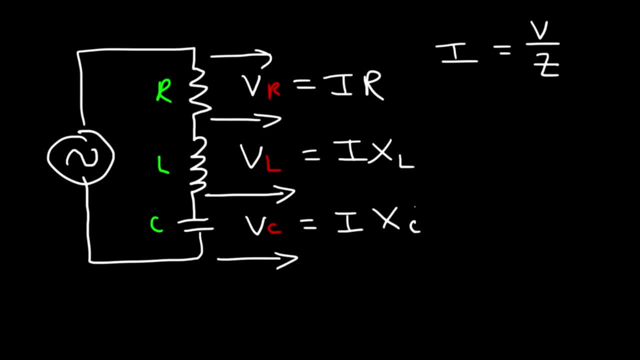 XL is the inductive reactance, which is also in ohms XC. the capacitive reactance is in ohms Z connects R, XL and XC together, as we've seen in this equation. So Z is a type of. it has the same unit of resistance. 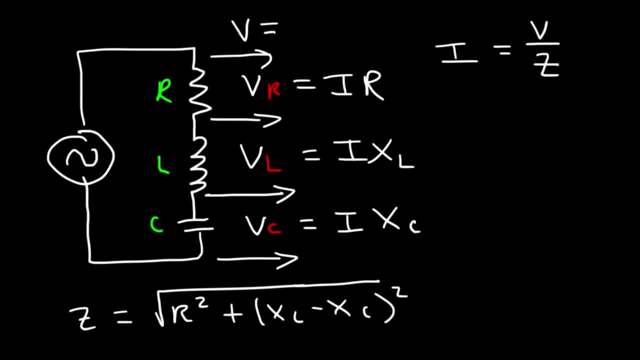 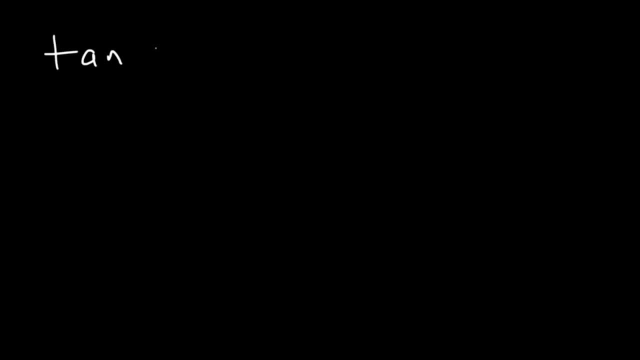 So, just as V equals Ir, V is equal to Iz. So that's how you can find the total current in the circuit. Just take the voltage, divide it by the impedance. Now there are some other equations that you need to know. So if you want to find the phase angle, 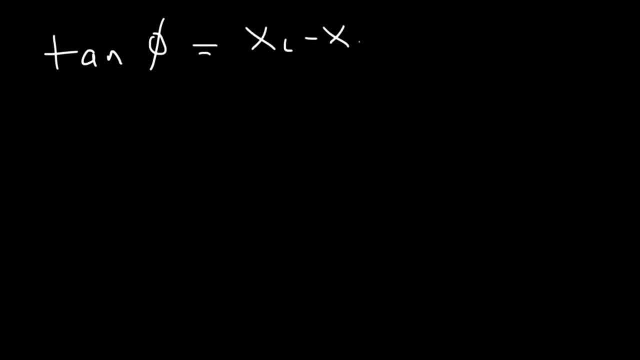 it's XL minus XL minus XC over R. Well, tangent of the phase angle, And the phase angle is going to be the arc tan of the inductive reactance minus the capacitive reactance over the resistance. You can also use this equation. 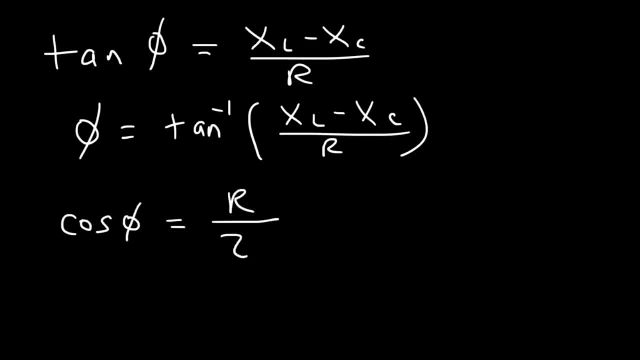 Cosine of the phase angle is equal to the resistance divided by the impedance. Cosine of the phase angle is also known as the power factor. Now, to calculate the power dissipated by the circuit, it's equal to I squared times R. Keep in mind: only the resistor dissipates energy. 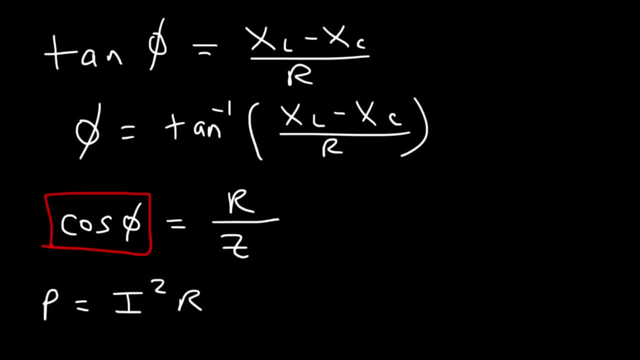 The inductor and capacitor. they both temporarily store it and then release it. So the power that is absorbed by the circuit is I squared R. You can also use this equation. It's equal to the. the average power is the Irms. 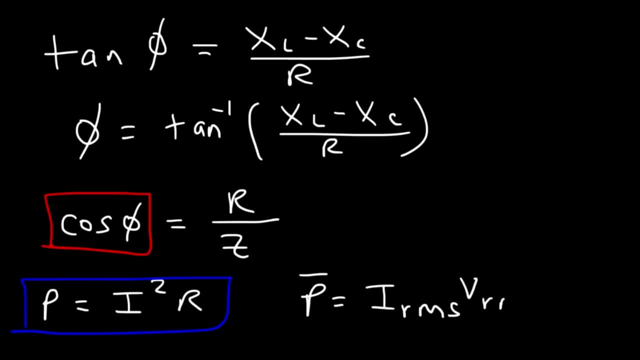 current and the voltage. RMS value times the power factor. So you can also calculate the average power using that formula, And that's basically it. These are the main formulas that you need to know for the RL circuit, the RC circuit and the RLC circuit. 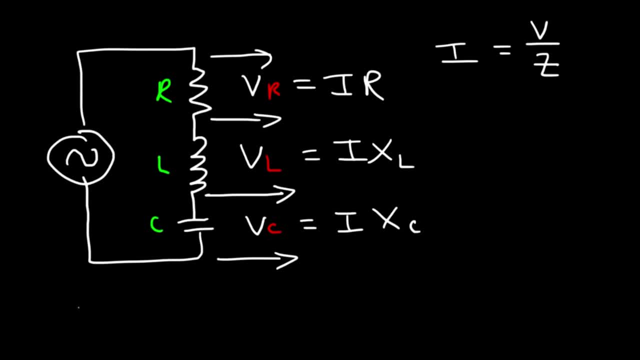 Z connects R, XL and XC together, as we've seen in this equation. So Z is a type of. It has the same unit of resistance. So, just as V equals IR, V is equal to IZ. So that's how you can find the total current in the circuit. 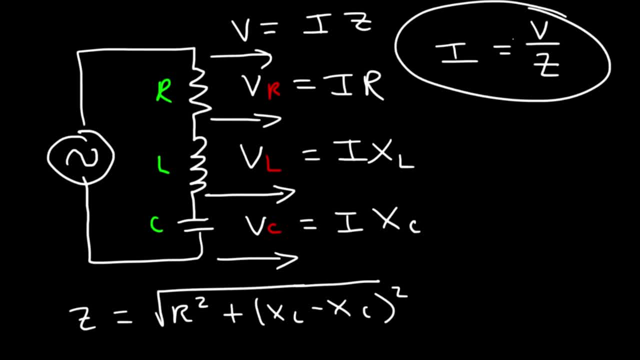 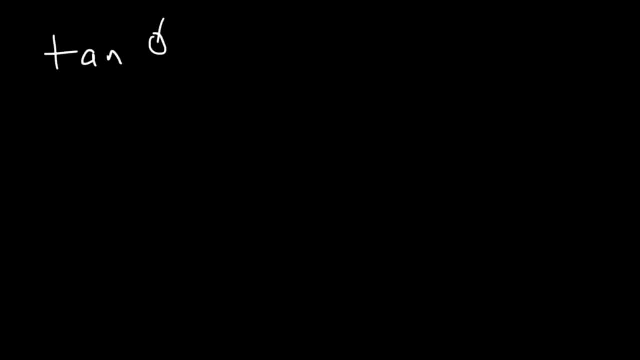 Just take the voltage, divide it by the impedance. Now there are some other equations that you need to know. So if you want to find the phase angle, it's XL minus XC over R, well, tangent of the phase angle. 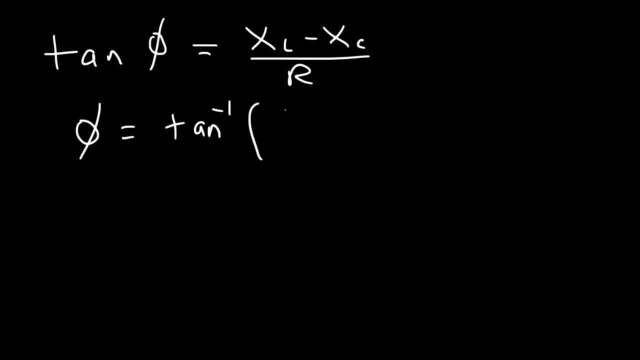 And the phase angle is going to be the arc tan of the inductive reactance minus the capacitive reactance over the resistance. You can also use this equation: Cosine of the phase angle is equal to the resistance divided by the impedance. Cosine of the phase angle is also known as the power factor. 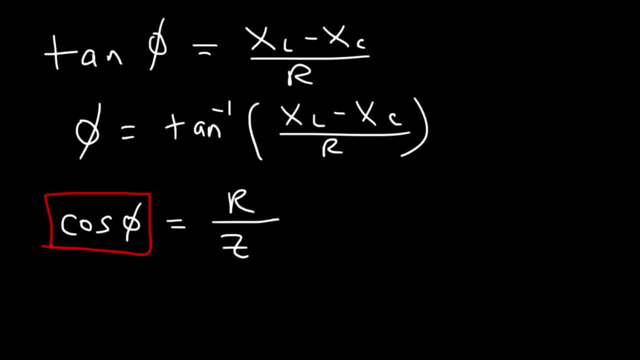 Now to calculate the power dissipated by the circuit. it's equal to I squared times R. Keep in mind: only the resistor dissipates energy, The inductor and capacitor. they both temporarily store it and then release it. So the power that is absorbed by the circuit is I squared R. 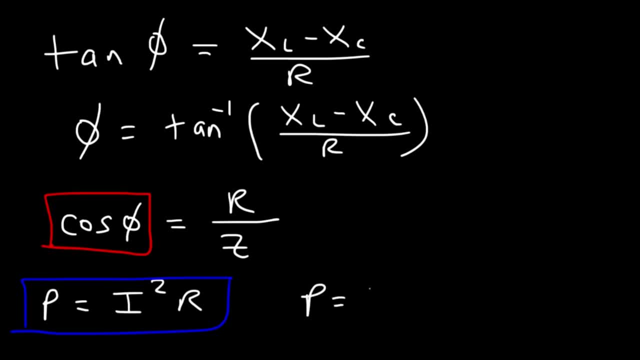 You can also use this equation. It's equal to the. The average power is the RMS current and the RMS is the current. So it's equal to the voltage RMS value times the power factor. So you can also calculate the average power using that formula. 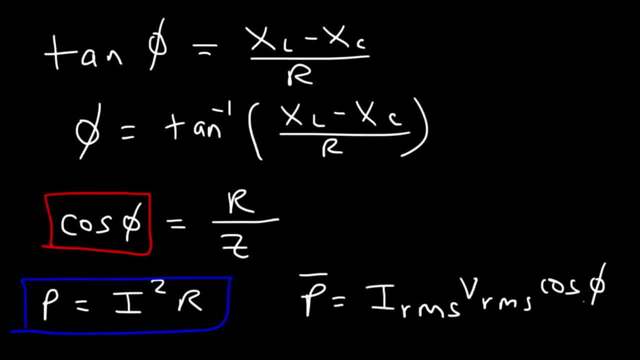 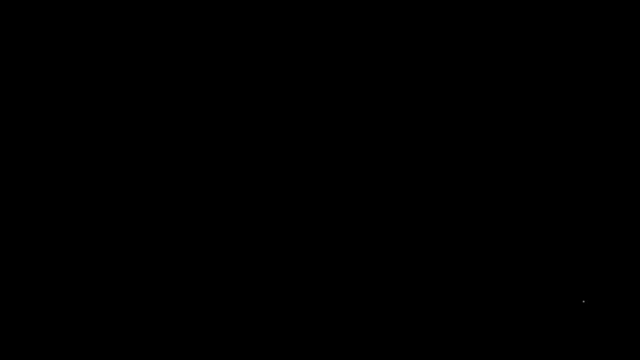 And that's basically it. These are the main formulas that you need to know for the RL circuit, the RC circuit and the RLC circuit. Now, whenever you have a circuit with a capacitor and an inductor, be it an LC circuit. 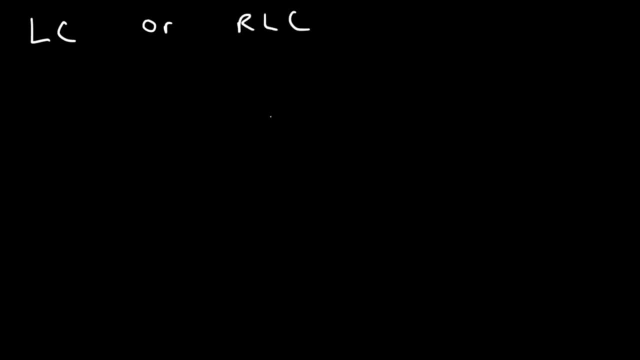 or an RLC circuit, you can calculate the resonant frequency, which is 1 over 2 pi square root LC. At the resonant frequency the capacitive reactants and the inductive reactants are equal to each other. So in that case, 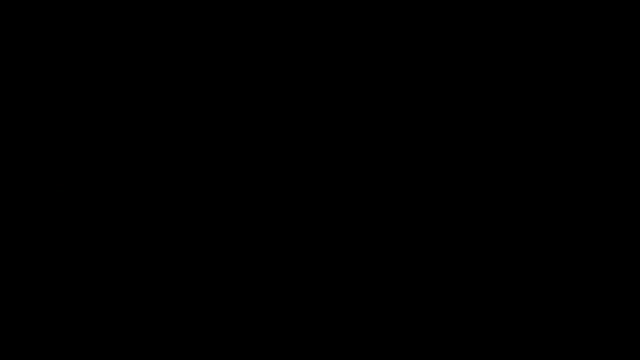 Now, whenever you have a circuit with a capacitor and an inductor, be it an LC circuit or an RLC circuit, you can calculate the resonant frequency, which is 1 over 2 pi square root LC At the resonant frequency. 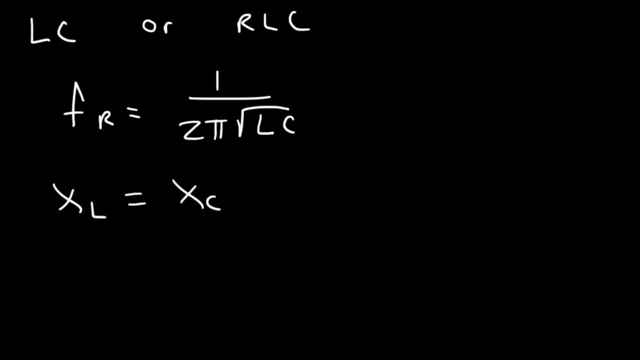 the capacitive reactants and the inductive reactants are equal to each other. So in that case, the impedance which is the square root of R squared plus xL minus xC, squared, since xL minus xC are the same, 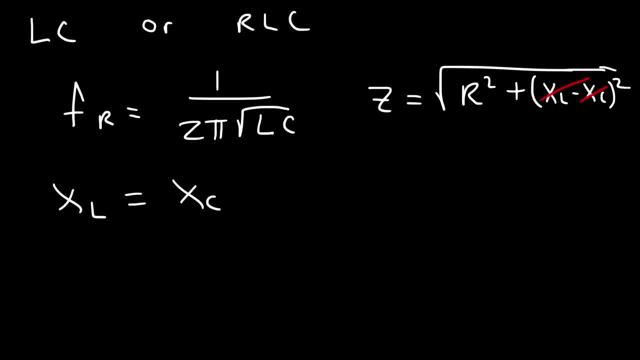 these two will cancel. xL minus xC is 0.. So Z is equal to R. So at the resonant frequency, make sure you know that capacitive reactants equal inductive reactants, xC equals xL and Z. the impedance is just the resistor. 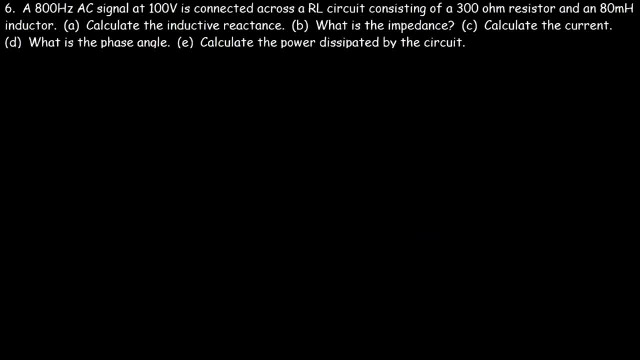 the resistance of the resistor Number 6.. A 800 Hz AC signal at 100 volts is connected across an RL circuit consisting of a 300 ohm resistor and an 80 mH inductor. Calculate the inductive reactants. So let's draw the circuit first. 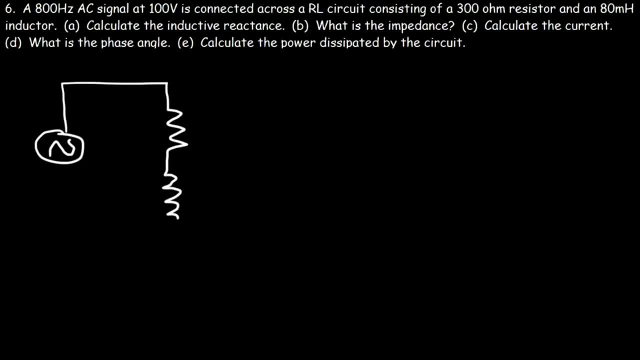 So we have a resistor and an inductor. So the frequency of the signal is 800 Hz And the voltage is 100 volts. Now we have a 300 ohm resistor and an 80 mH inductor. So to find the inductive reactants. 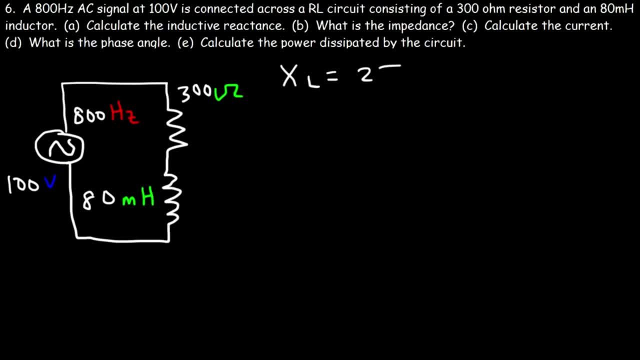 we can use this equation: xL is equal to 2 pi fL, So that's 2 pi times the frequency of 800 times L, 80 mH, or 80 times 10 to the minus 3.. If you see milli. 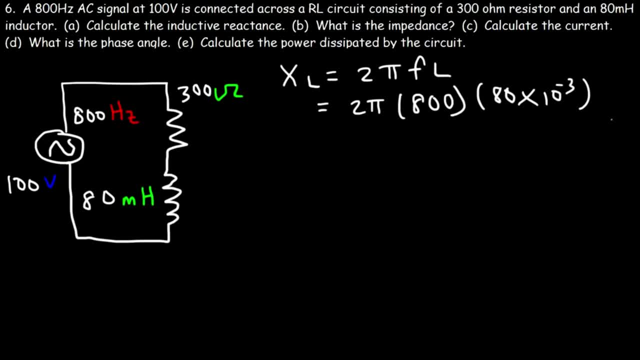 you could just add 10 to the negative 3 to it. That's a quick way to convert it. So xL is equal to 402, is equal to 402 ohms or 402.1 ohms. Now let's calculate the impedance. 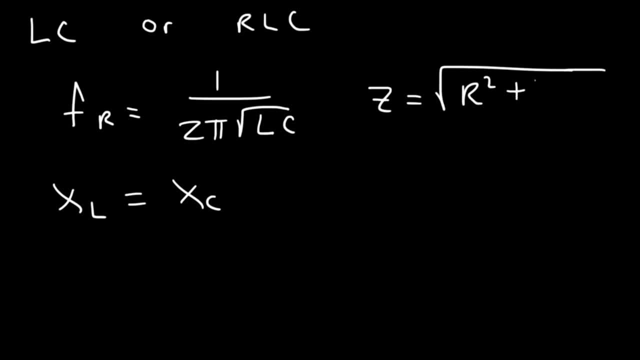 the impedance, which is the square root of R squared plus XL minus XC squared. Since XL minus XC are the same, these two will cancel. XL minus XC is zero, So Z is equal to R. So at the resonant frequency, 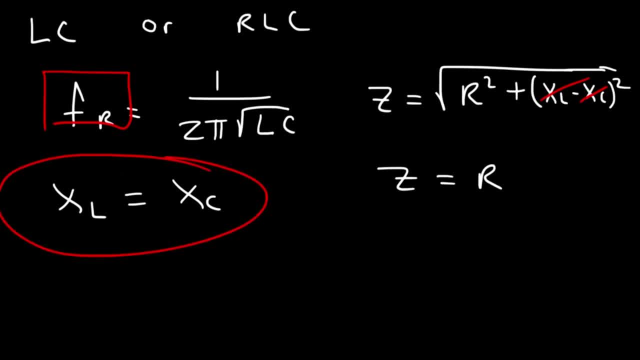 make sure you know that capacitive reactants equal inductive reactants, XC equals XL And Z. the impedance is just the resistor. the resistance of the resistor Number six: A 800 Hertz ACC. a 100 Hertz ACC. signal at 100 volts. 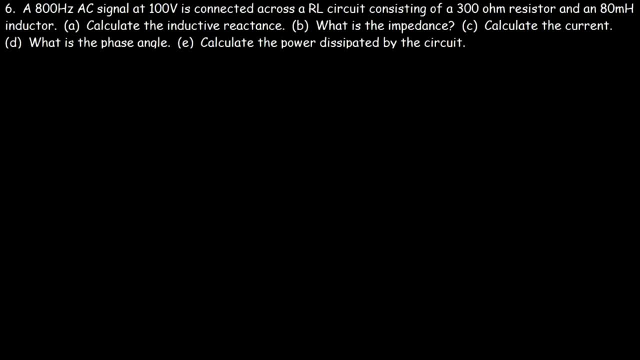 is connected across an RL circuit consisting of a 300 ohm resistor and an 80 milliHenry inductor. Calculate the inductive reactants, So let's draw the circuit first. So we have a resistor and an inductor. 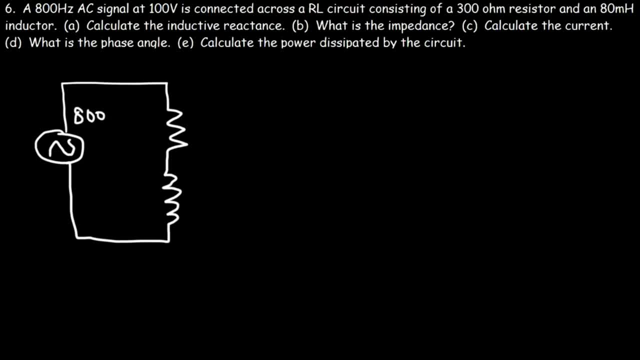 So the frequency of the signal is 800 Hertz And the voltage is 100 volts. Now we have a 300 ohm resistor and an 80 milliHenry inductor. So to find the inductive reactants. 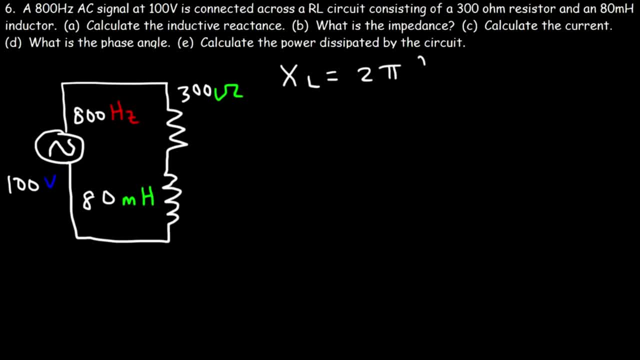 we can use this equation: XL is equal to two pi FL. So that's two pi FL. So that's pi times the frequency of 800 times L, 80 milliHenrys or 80 times 10 to the minus three. 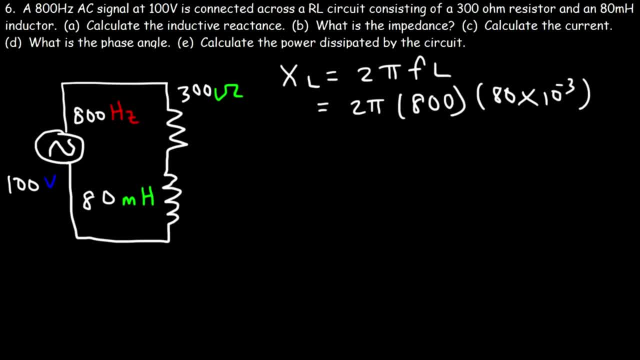 If you see milli, you could just add 10 to negative three to it. That's a quick way to convert it. So XL is equal to 402 ohms or 402.1 ohms. Now let's calculate the impedance. 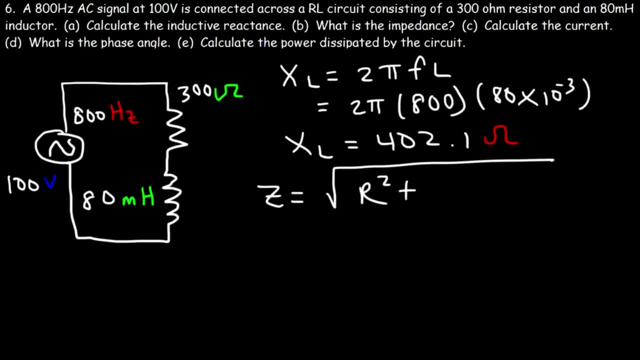 The impedance is gonna be the square root of R squared plus XL minus XC squared. Since there's no capacitor in the circuit, XC is zero. So R- the resistor has a value of 300 ohms, and XL is 402.1.. 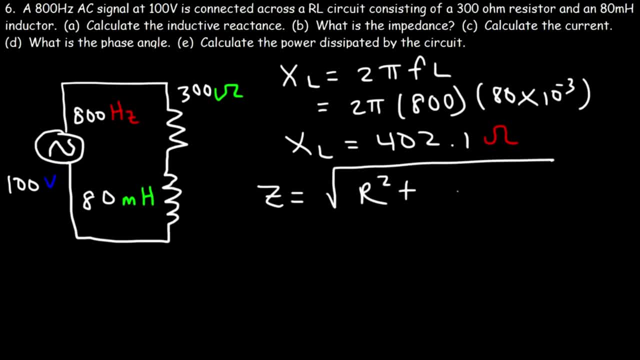 The impedance is going to be the square root of R squared plus xL minus xC squared. Since there's no capacitor in the circuit, xC is 0.. So R, the resistor, has a value of 300 ohms And xL is 402.1.. 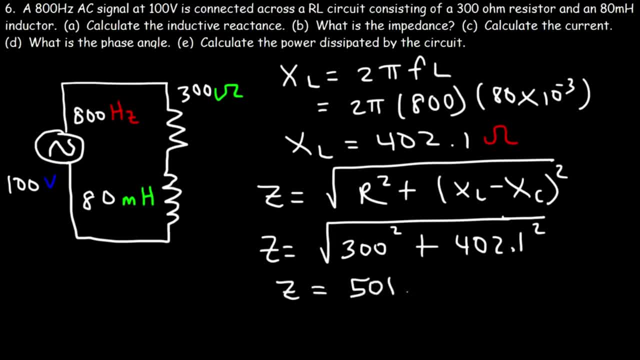 So the impedance of the circuit is 501.7 ohms. Now let's move on to part C. What is the current in the circuit? To find the current, it's simply equal to the voltage divided by the impedance. The voltage is 100 volts. 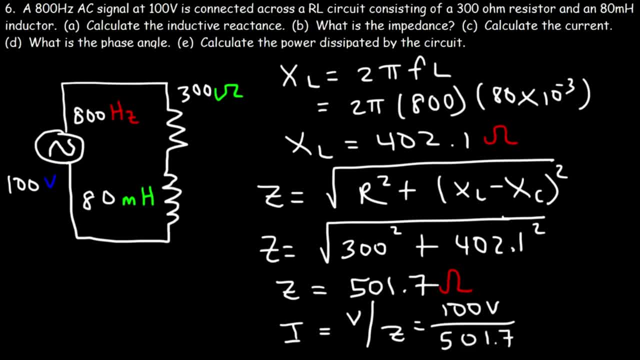 The impedance is 501.7 ohms, So this is equal to 0.199 amps. So that's the current in the circuit. Now what about part D? What is the phase angle? To calculate the phase angle, we can use this equation: 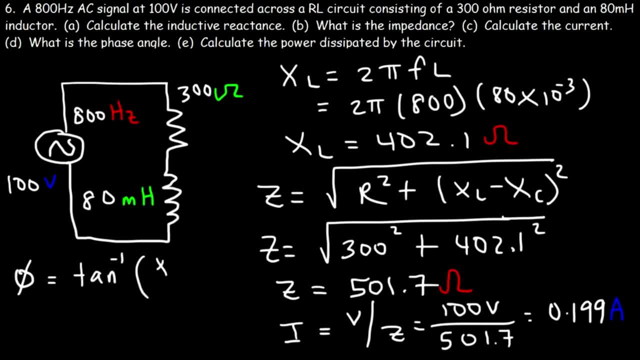 Arc tan xL minus xC over R. So in this case xL, we can see that it's 402.1.. xC is 0.. And R that's 300 ohms. So arc tan 402.1 divided by 300. 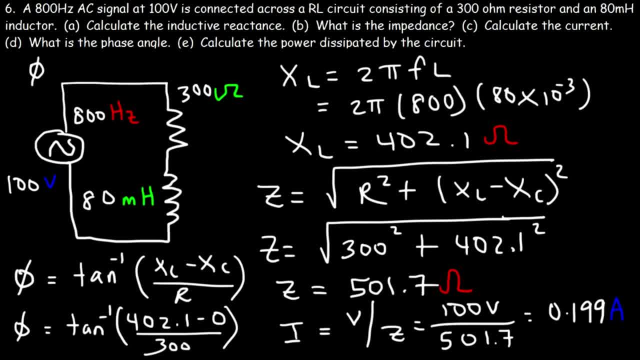 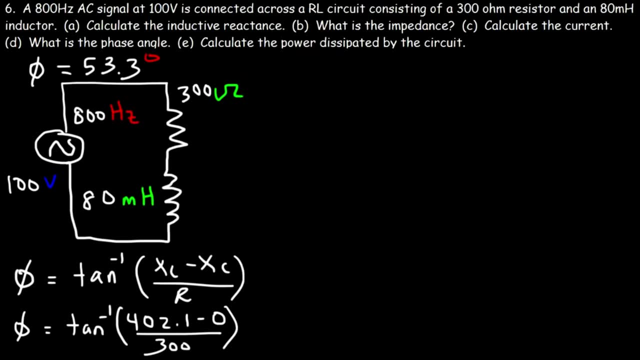 Make sure your calculator is in degree mode. by the way, This will give you a phase angle of 53.3 degrees. Now there's another way in which we can calculate the phase angle. We can use this formula as well. It's equal to the arc cosine. 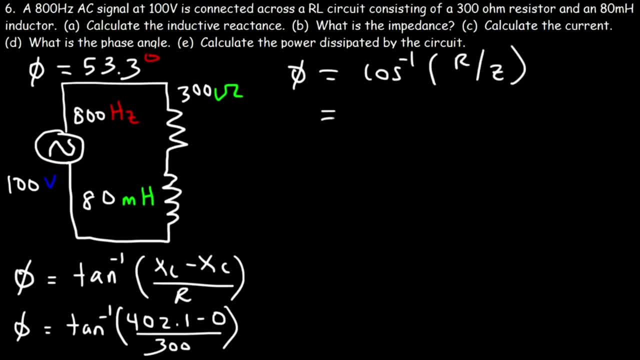 of R divided by Z. So the resistance is 300 and the impedance that was 501.7.. I believe that was the number that I used before. So if you type in arc cosine 300 divided by 501.7,, this will give you the same answer. 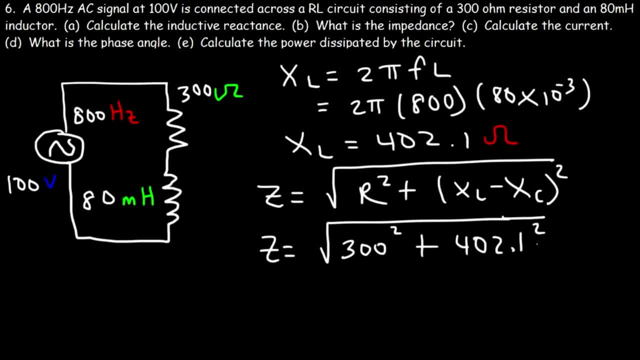 So the impedance of the circuit is 501.7 ohms. Now let's move on to part C. What is the current in the circuit? To find the current, it's simply equal to the voltage divided by the impedance. The voltage is 100 volts. 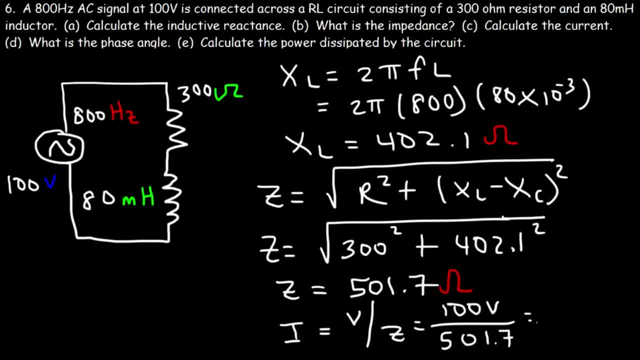 The impedance is 501.7 ohms, So this is equal to 0.199 amps. So that's the current in the circuit. Now what about part D? What is the phase angle? To calculate the phase angle, we can use this equation: 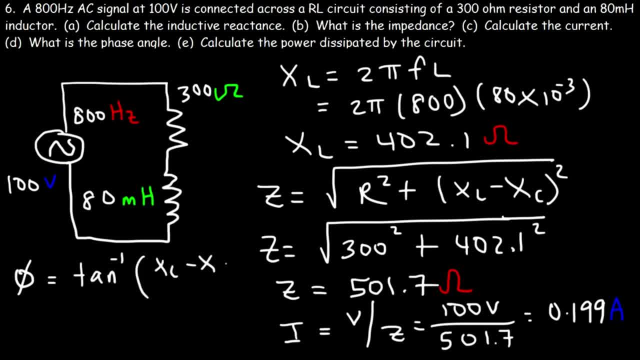 R tan XL minus XC over R. So in this case XL, we can see that it's 402.1.. XC is zero and R that's 300 ohms. So R tan 402.1 divided by 300.. 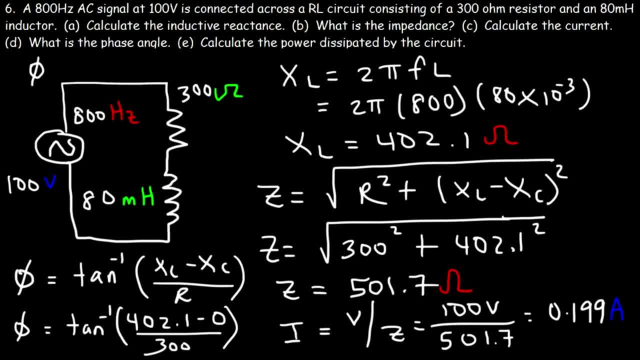 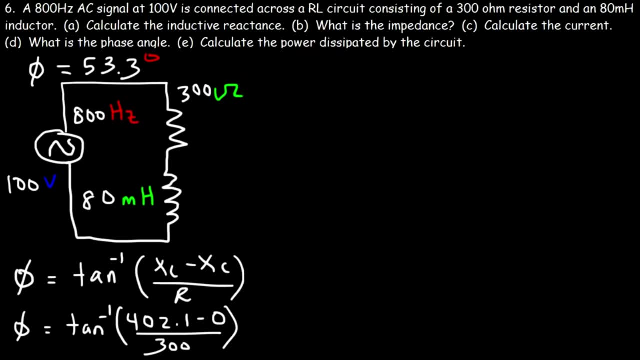 Make sure your calculator is in degree mode, by the way. This will give you a phase angle of 53.3 degrees. Now there's another way in which we can calculate the phase angle. We can use this formula as well. It's equal to the arc cosine of R divided by Z. 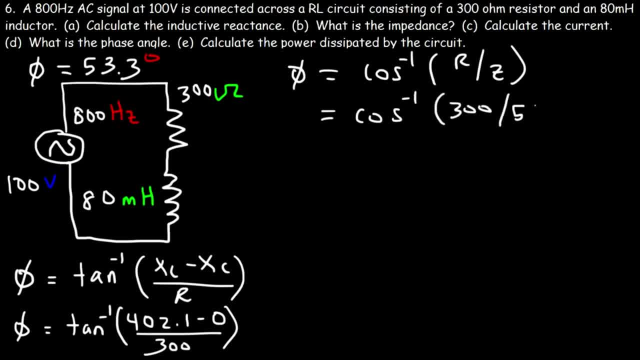 So the resistance is 300, and the impedance that was 501.7.. I believe that was the number that I used before. So if you type in arc cosine, 300 divided by 501.7,, this will give you the same answer of 53.3 degrees. 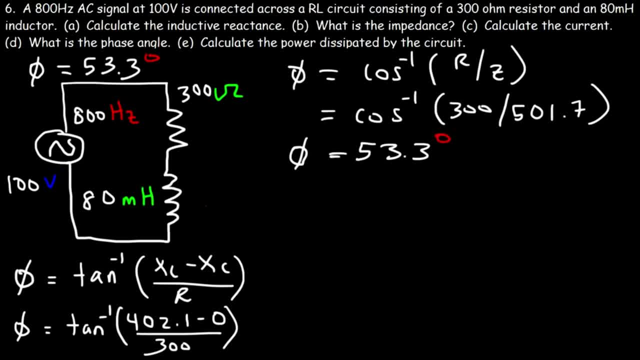 So that's the phase angle. Now what about part E? Calculate the power dissipated by the circuit. A simple way to do that is to use the formula. So that's the phase angle. Now what about part E: Calculate the power dissipated by the circuit.